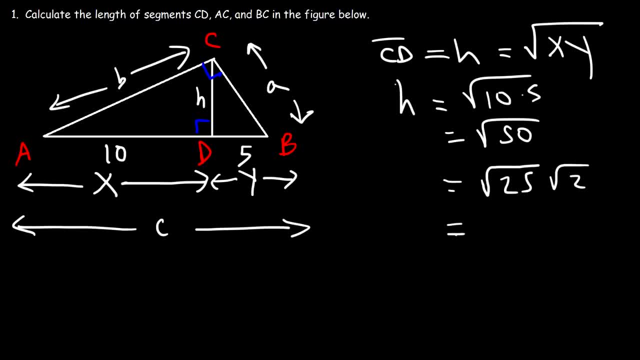 to break down 50 into 25 and 2.. Now the square root of 25 is 5.. So the exact answer for H, which is segment CD, is 5, square root 2.. So that's the length of the altitude. Now let's. 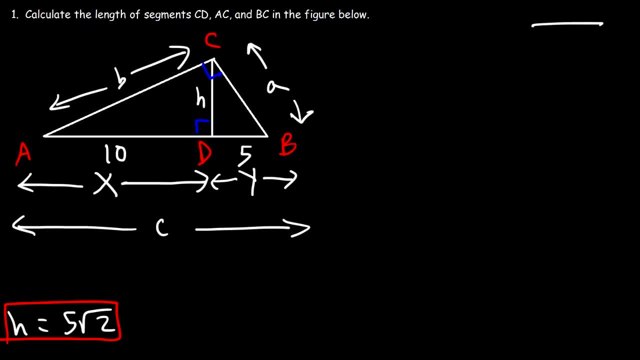 calculate the next segment, and that is segment AC. Segment AC is represented by B in the equation. Now how can we calculate B? B is the geometric mean between X and C, So B is the square root of X times C. In this example, X is the. 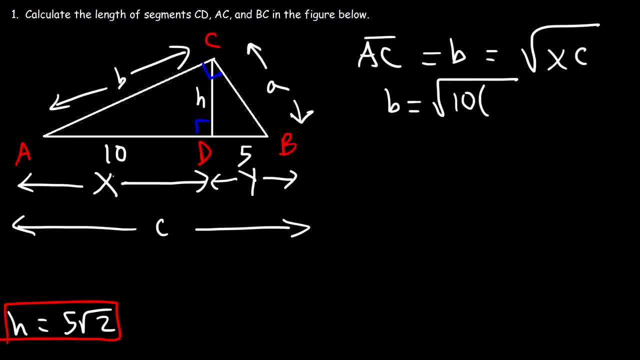 10, and C is the sum of X and Y. So C is the sum of 10 and 5,, which is 15.. So 10 times 15 is 150.. Now how can we simplify this? radical 25 can go into 150. In fact, 150 is 25 times. 6. To get the 6, just take 150 and multiply it by 6.. Now how can we simplify this? radical 25 can go into 150. In fact, 150 is 25 times 6.. To get the 6, just take 150. 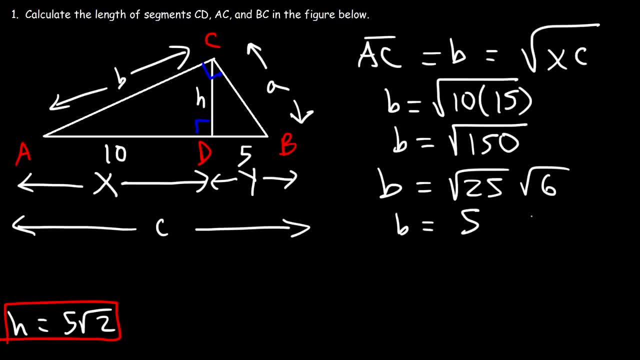 and divide it by 26.. Now the square root of 25, we know it's 5.. So B, which represents segment AC, that's equal to 5, square root 6.. So that's the second answer. Now let's move on to the next part, and that is the length of BC. 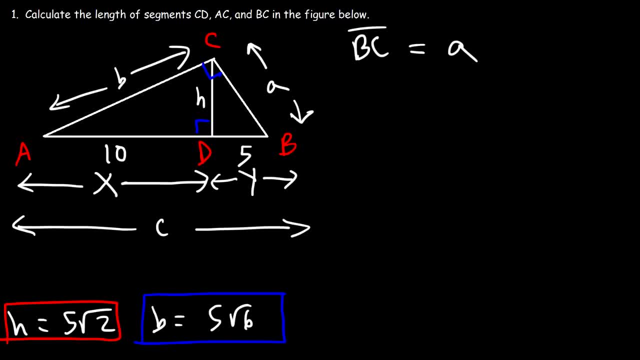 So segment BC is equal to A. Now what do you think A is going to be? the geometric mean of A is the geometric mean of Y and C. So A is equal to the square root of Y times C. So Y is 5 and C, just like before, is the sum of X and Y. 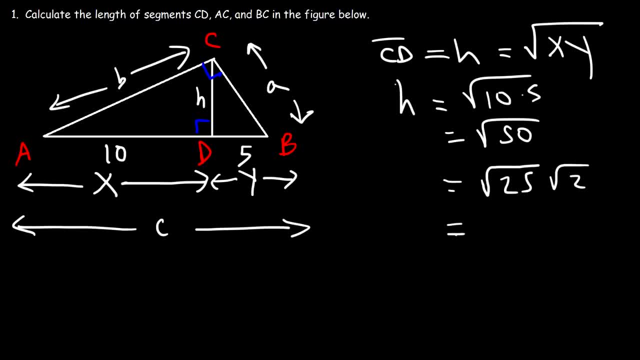 to break down 50 into 25 and 2.. Now the square root of 25 is 5.. So the exact answer for H, which is segment CD, is 5, square root 2.. So that's the length of the altitude. Now let's. 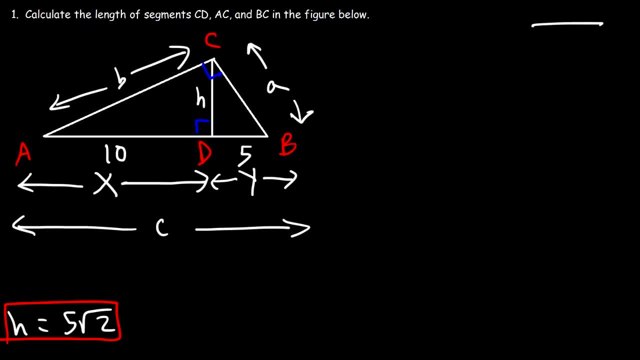 calculate the next segment, and that is segment AC. Segment AC is represented by B in the equation. Now how can we calculate B? B is the geometric mean between X and C, So B is the square root of X times C. In this example, X is the. 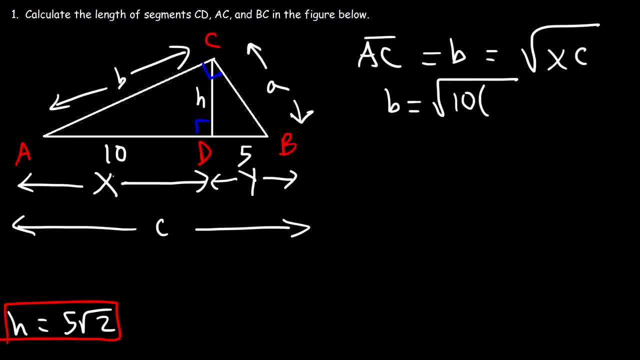 10, and C is the sum of X and Y. So C is the sum of 10 and 5,, which is 15.. So 10 times 15 is 150.. Now how can we simplify this? radical 25 can go into 150. In fact, 150 is 25 times. 6. To get the 6, just take 150 and multiply it by 6.. Now how can we simplify this? radical 25 can go into 150. In fact, 150 is 25 times 6.. To get the 6, just take 150. 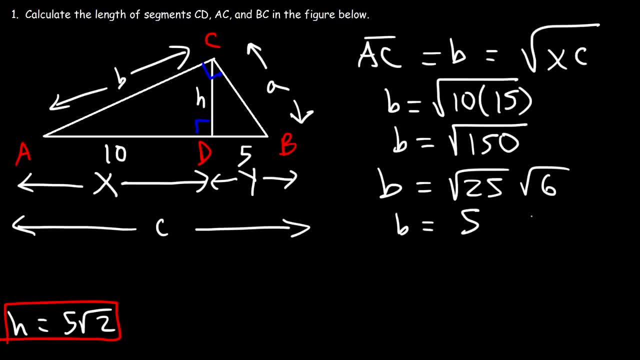 and multiply it by 26.. Now the square root of 25, we know it's 5.. So B, which represents segment AC, that's equal to 5, square root 6.. So that's the second answer. Now let's move on to the next part, and that is the length of BC. 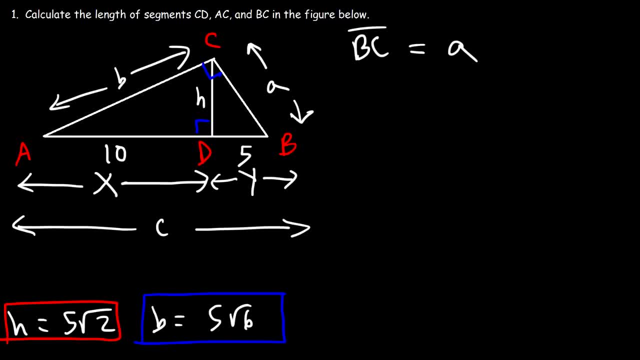 So segment BC is equal to A. Now what do you think A is going to be? the geometric mean of A is the geometric mean of Y and C. So A is equal to the square root of Y times C. So Y is 5 and C, just like before, is the sum of X and Y. 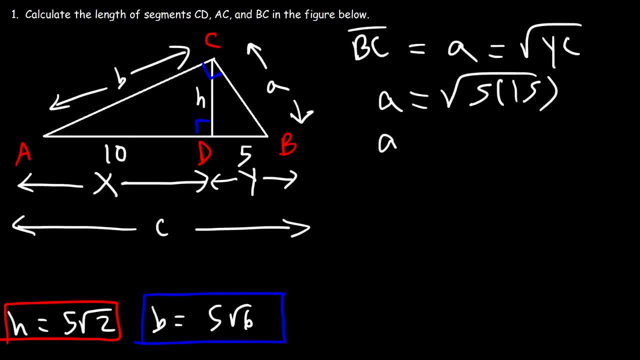 And so C is 15, just like before. Now, 5 times 15 is 75, and 75 is 25 times 3, and we know the square root of 25 is 5.. So A is 5, square root 3.. 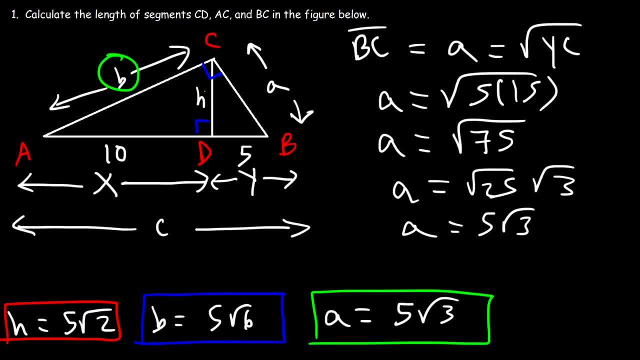 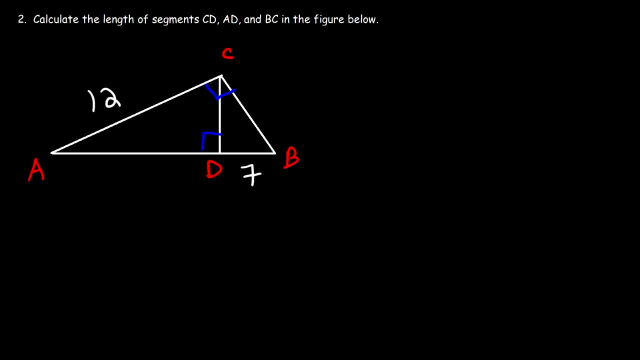 And so that's how you can calculate the length of segment AC, DC and BC, Given AD and BC And BD. So that's it for this problem Number 2.. Calculate the length of segments CD, AD and BC in the figure below. 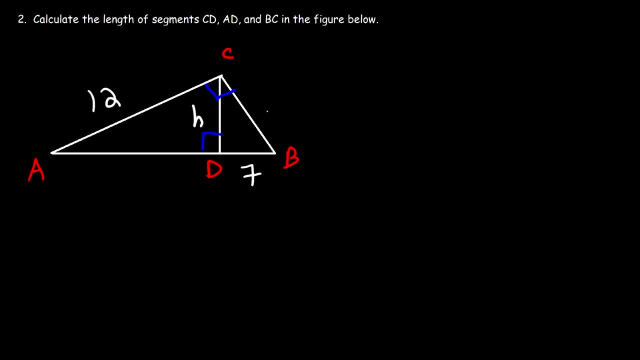 So CD is H, AD is X and BC is opposite to angle A. So that's A. Opposite to angle B is side B, Opposite to angle B is side B And opposite to angle C is side C. Now we know DB is Y and AD is X, which is equal to X in this example. 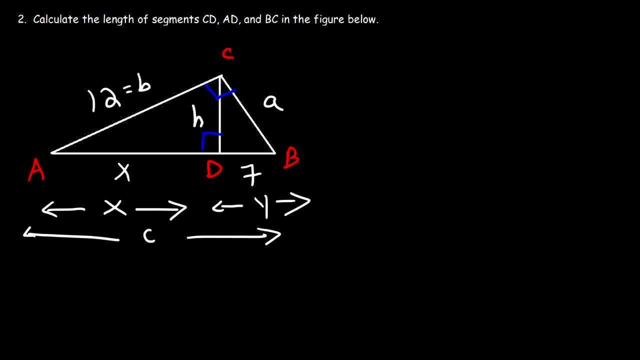 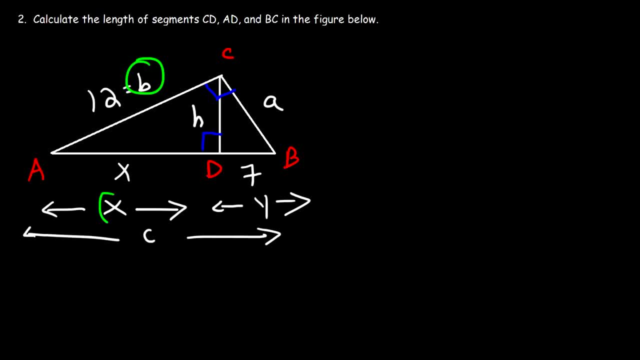 B is the geometric mean between X and C, So B is the square root of X and C. H is the geometric mean between X and Y, So H is the square root of X times Y, And A is the geometric mean between Y and C. 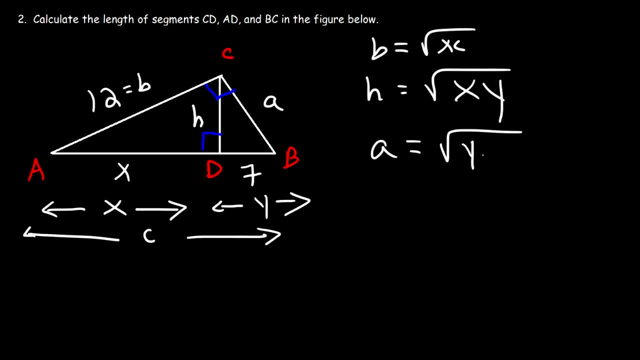 So A is the square root of X times Y, And B is the square root of Z times Y, And C is the geometric mean between B and Z, Loading on the shapes between A and Z. Another thing to consider is that when you're 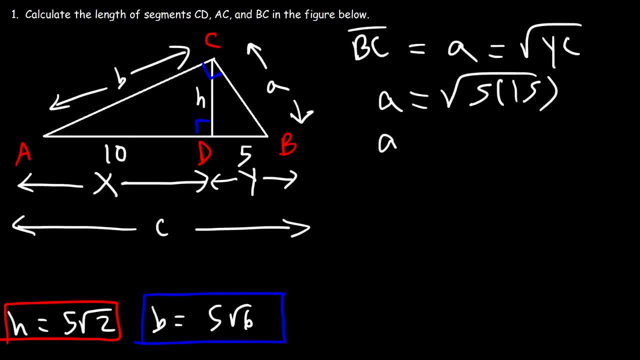 And so C is 15, just like before. Now, 5 times 15 is 75, and 75 is 25 times 3, and we know the square root of 25 is 5.. So A is 5, square root 3.. 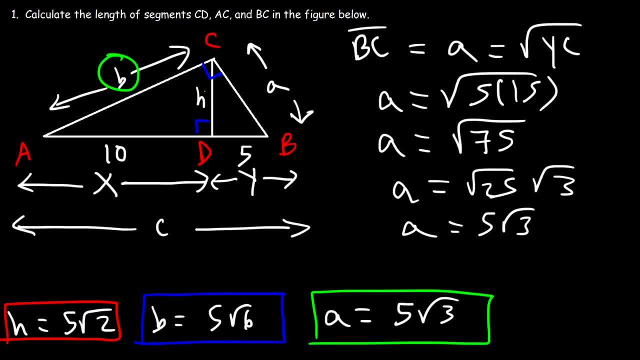 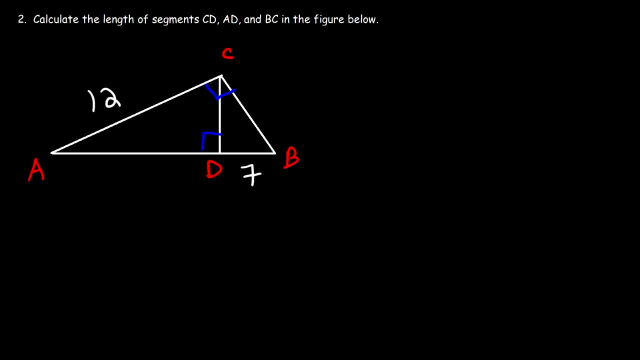 And so that's how you can calculate the length of segment AC, DC and BC, Given AD and BC And BD. So that's it for this problem Number 2.. Calculate the length of segments CD, AD and BC in the figure below. 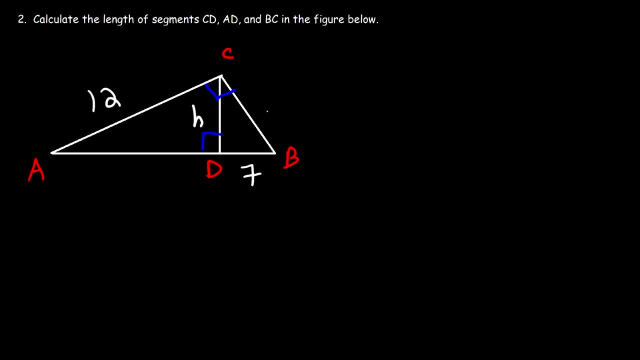 So CD is H, AD is X and BC is opposite to angle A. So that's A. Opposite to angle B is side B, Opposite to angle B is side B And opposite to angle C is side C. Now we know DB is Y and AD is X, which is equal to X in this example. 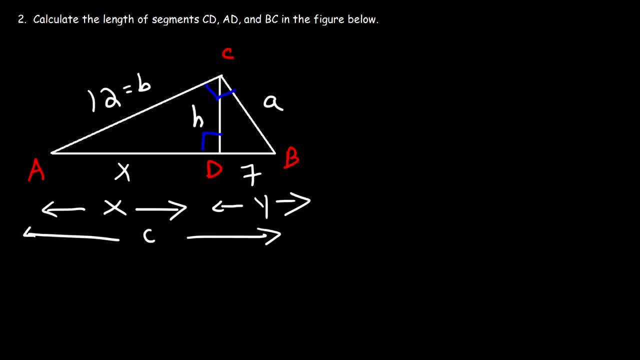 So which one should we calculate first? Segment CD, AD or BC? Should we try to calculate X, H or A first? Now let's go over the equations. B is X, H or A first? Now let's go over the equations. 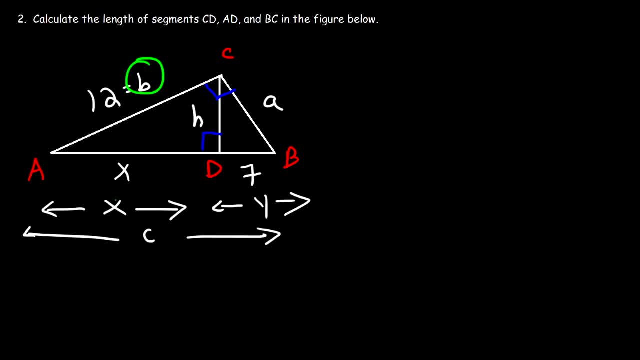 B is X, H or A first. Now let's go over the equations: B is X, H or A first. First line: A is the geometric mean between X and C. G is the geometric mean between X and C. 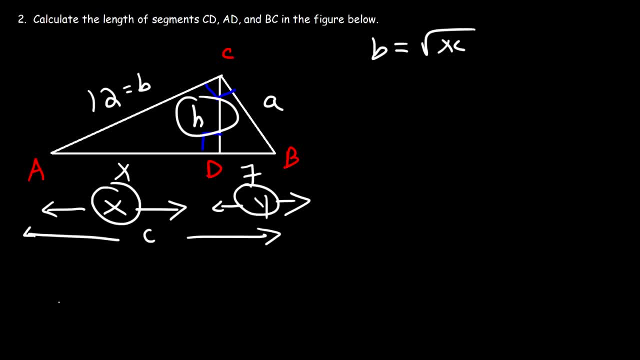 H is the geometric mean between X and Y. So H is the square root of X times Y and A is the geometric mean between Y and C. so A is the square root of X times Y is quierex and C square root of Y times C. Make sure you remember these three equations because they can help. 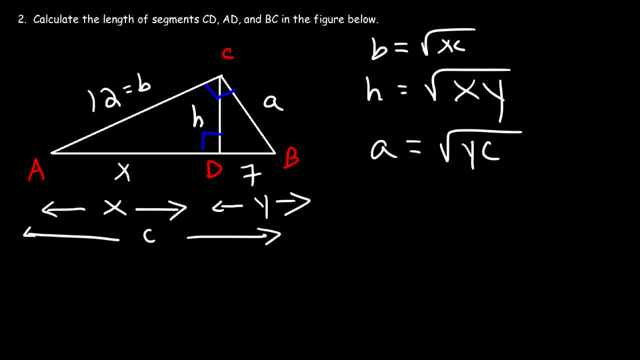 you to solve what you're looking for in this particular problem. So the issue that we're faced with in this problem is deciding which letter we should calculate first- A, H or X. Well, let's pick one. Let's start with A. 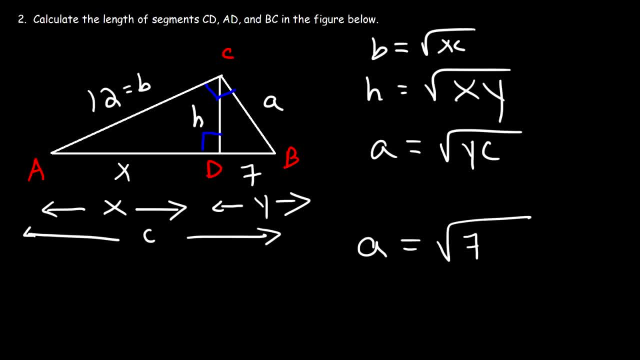 So A is equal to the square root of Y, which is 7,, and C is the sum of X and Y. So X in this problem is just X, Y is 7.. So C is X plus 7.. So this formula is not going to be helpful because we have two variables that we don't. 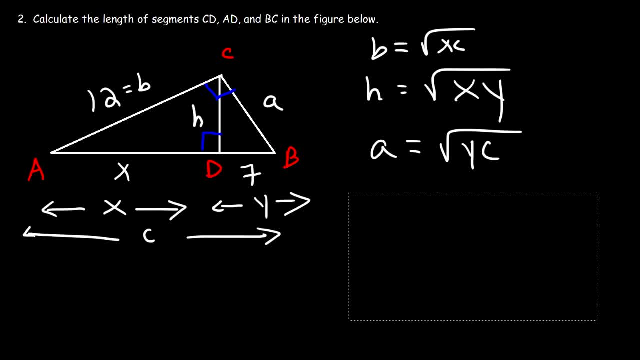 know the value of currently. So let's get rid of this. Let's try the second one, H. So H is the square root of XY. We don't know X, but we know Y is 7.. We still have two unknowns. 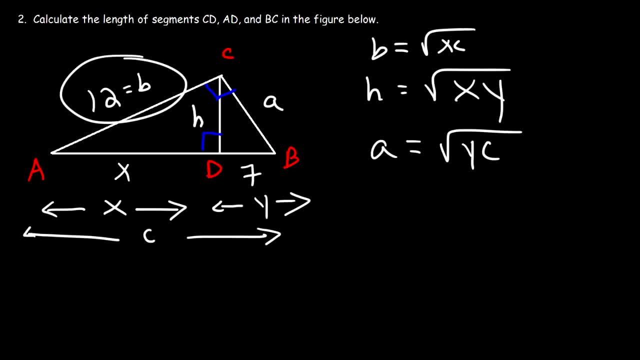 So now let's try B. We do have the value of B. B is 12,, X is X and C is X plus 7.. So in this equation we only have one variable. So now this is where we should start. 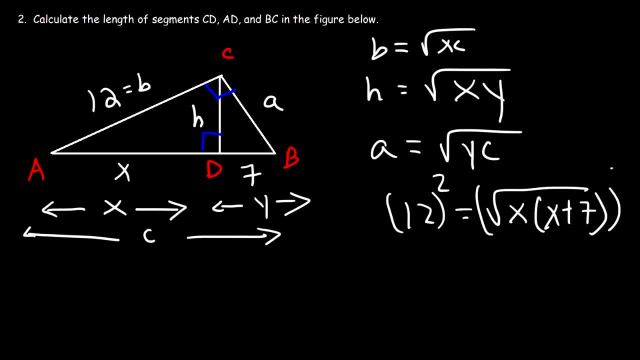 So let's square both sides to get rid of the square root. So 12 squared is 144.. So 12 squared is 144. And when we square the square root, those two will cancel. And so we're left with X times X plus 7.. 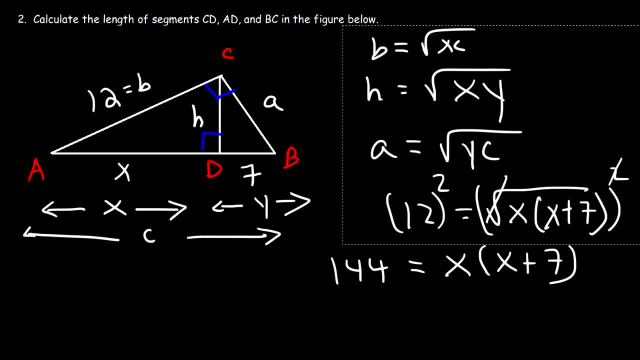 So now, what do we need to do at this point? in order to solve it Right now, we need to distribute X. So X times X is X squared, and X times 7 is 7X. Let's take the 144 and move it to this side. 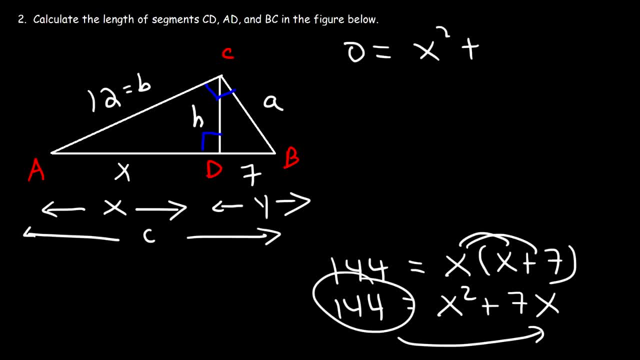 So 0 is equal to X squared plus 7.. So 0 is equal to X squared plus 7X minus 144.. Now we need to find two numbers that multiply to negative 144, but add to positive 7.. So what are those two numbers? 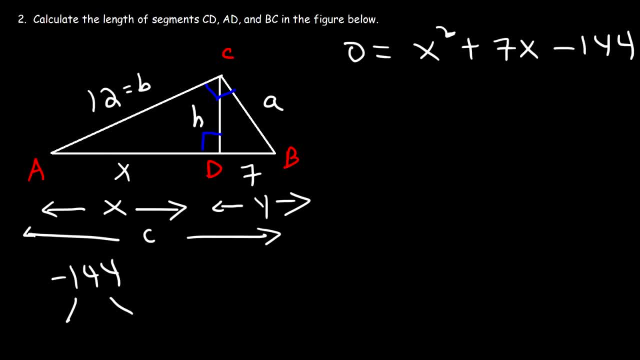 Well, let's make a list. Since the list might be somewhat big, I'm going to do it on the right side. So we need the sum to be positive. So we need the sum to be positive. So we need the sum to be positive. calculating the X and Y values estaba ayudando al esc. The value of the Y all ended in: Do these know their school? Yes, Good luck every one. Thanks, Let's pick one. Let's start with A. A is equal to the square root of Y, which is 7.. 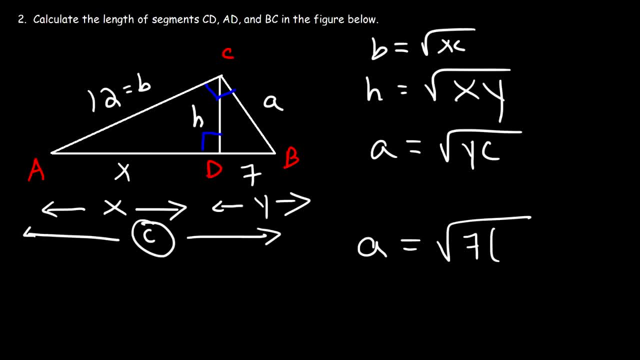 x and y. So x in this problem is just x, y is 7.. So c is x plus 7.. So this formula is not going to be helpful because we have two variables that we don't know the value of currently. So let's get. 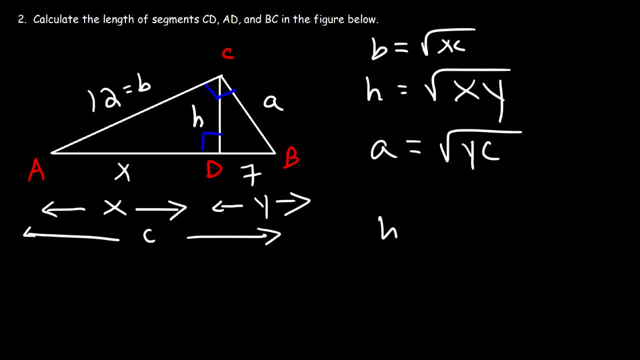 rid of this. Let's try the second one, h. So h is the square root of xy. We don't know x, but we know y is 7.. We still have two unknowns, So now let's try b. We do have the value of b. b is 12,. 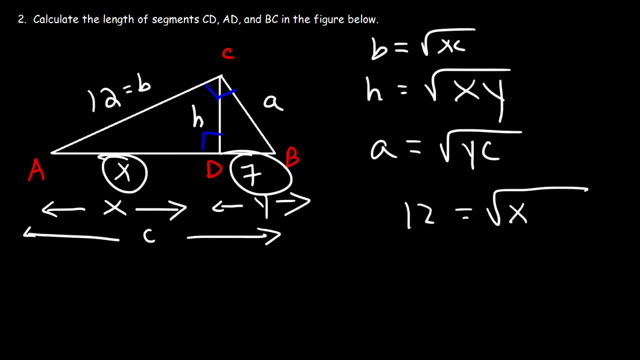 x is x and c is x plus 7.. So in this equation we only have one variable. So now this is where we should start. So let's square both sides to get rid of the square root. So 12 squared is 144, and when we square, 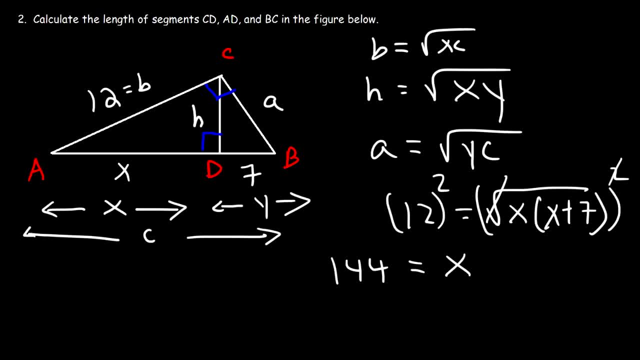 the square root, those two will cancel, And so we're left with x times x plus 7.. So now, what do we need to do at this point? in order to solve it Right now, we need to distribute x. So x times x is x squared, and x times 7 is 7x. Let's take the 144 and move it to this side. 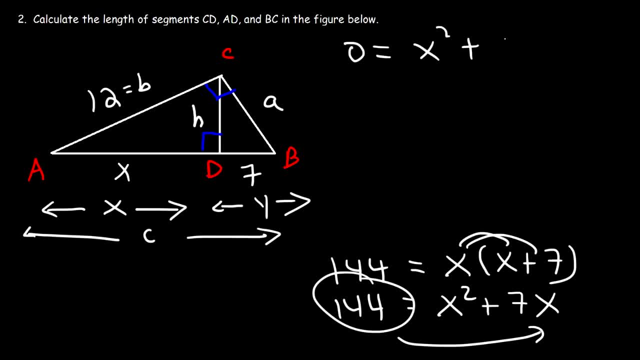 So 0 is equal to x squared plus 7x, 7x minus 144.. Now we need to find two numbers that multiply to negative 144 but add to positive 7.. So what are those two numbers? Well, let's make a list, Since the list might be. 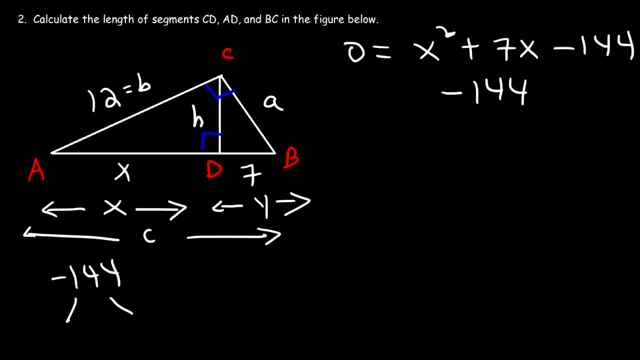 somewhat big. I'm going to do it on the right side, So we need the sum to be positive. So let's divide by a small negative number so we can get a large positive number. So if I divide by negative 2, this is going to be positive 72. Now these two numbers add up. 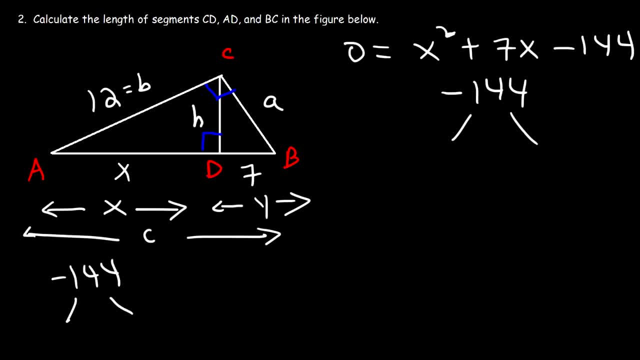 So let's divide by a small negative number so we can get a large positive number. So if I divide by negative 2, this is going to be positive 72. Now these two numbers add up to positive 70. So now let's move on to negative 3.. 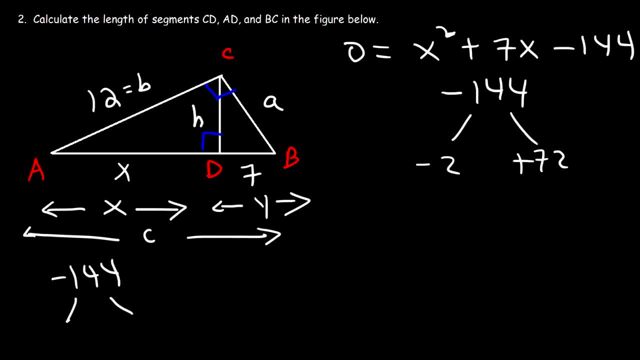 to positive 70.. So now let's move on to negative 3.. Negative 144 divided by negative 3 is positive 48. So these two differ by 45. So we're getting closer to 7,. so we're going in the right direction. 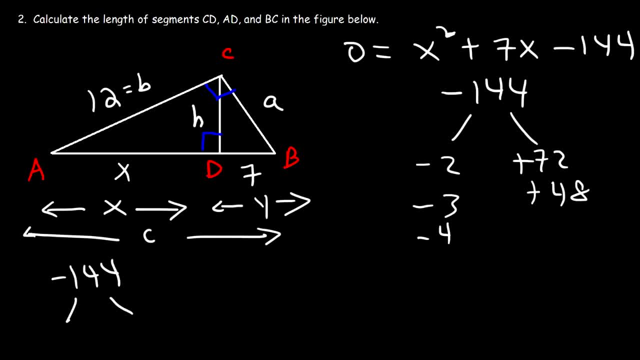 Let's divide by negative 4. This is positive 36. 5 doesn't go into 144.. Think of 144 as 12 times 12.. Since 5 doesn't go into 12, it's not going to go into 144.. Now we can try 6.. So this is: 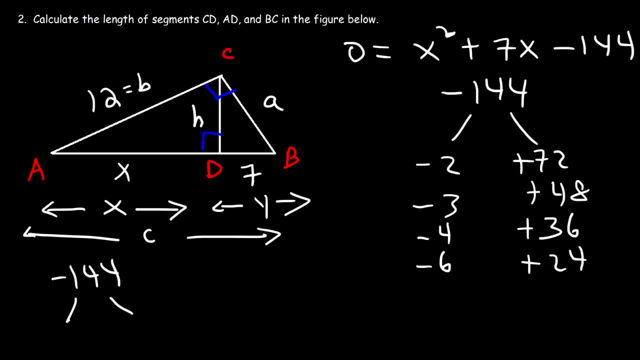 going to be positive 24.. And we could try. 8 goes into 24, so we could try that. And this is 18.. Now 9 goes into 36, so 9 goes into 144.. So negative 144 divided by negative 9 is: 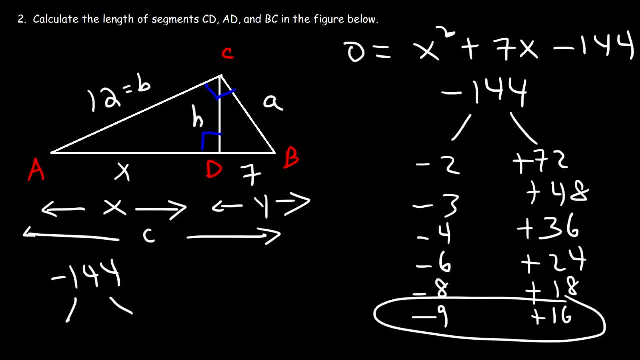 positive 16.. So notice that these two numbers add up to 7.. So now we can factor it, So it's going to be x minus 9 times x plus 16.. So if we set each factor equal to 0, we can see that x is equal to positive 9 and negative 16.. Now we can't use this. 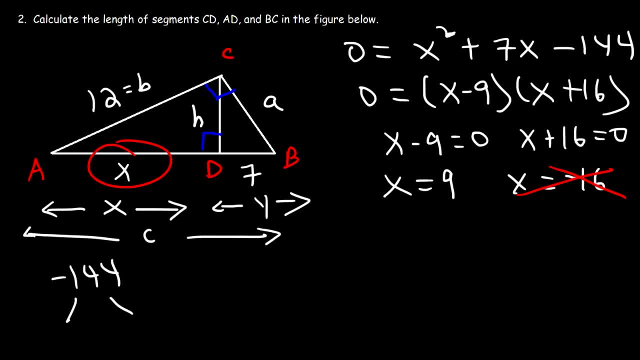 answer, because AD cannot be a negative side length, So therefore x has to be positive 9.. So now we know this value, This is 9.. So now we can calculate everything else, once we have these two values. So now let's calculate h. So we said that h is the geometric mean between x and y. 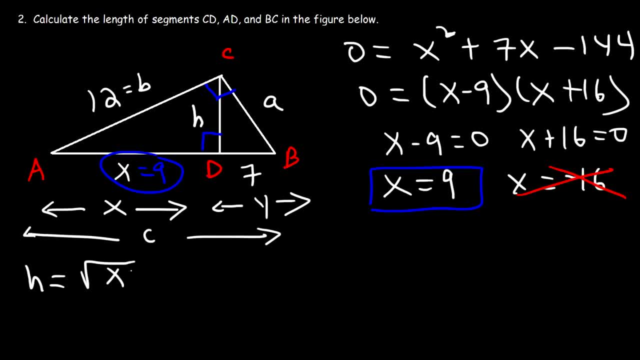 So it's the square root of x times y. So x is 9 and y is 7.. So 9 times 7 is 63, but we don't have to worry about that. We can take the square root of 9,, which is 3.. So 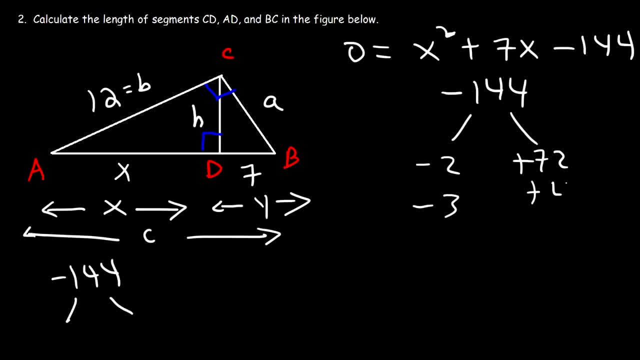 Negative 144, divided by negative 3 is positive 48. So these two differ by 45. So we're getting closer to 7, so we're going in the right direction. Let's divide by negative 4.. This is positive 36.. 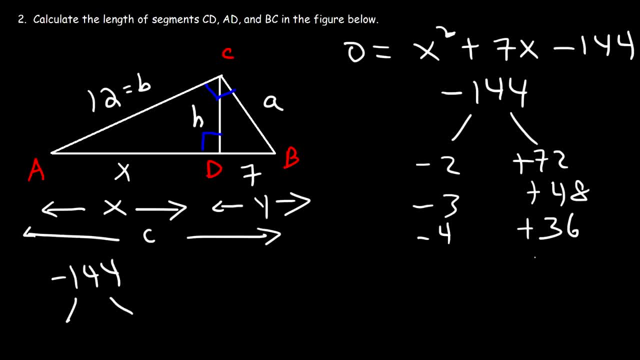 Five doesn't go into 144.. Think of 144 as 12 times 12.. Since 5 doesn't go into 12, it's not going to go into 144.. Now we can try 6.. So this is going to be positive 24.. 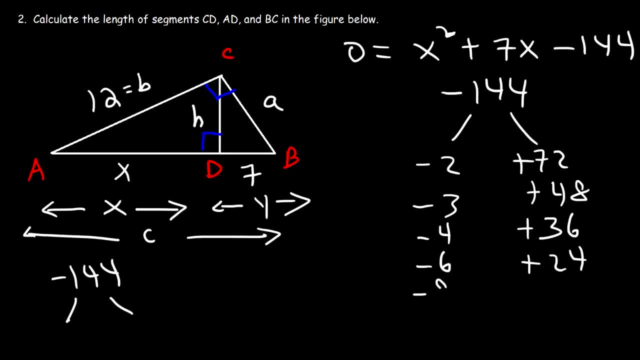 And we could try. 8 goes into 24, so we could try that. And this is 18.. Okay, So this is 18.. Now 9 goes into 36, so 9 goes into 144.. So negative 144 divided by negative 9 is positive 16.. 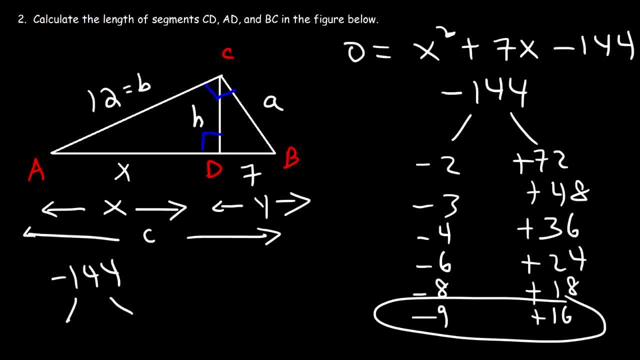 So notice that these two numbers add up to 7.. So now we can factor it, So it's going to be x minus 9 times x plus 16.. So if we set each factor equal to 0, we can see that x is equal to positive, 9 and negative. 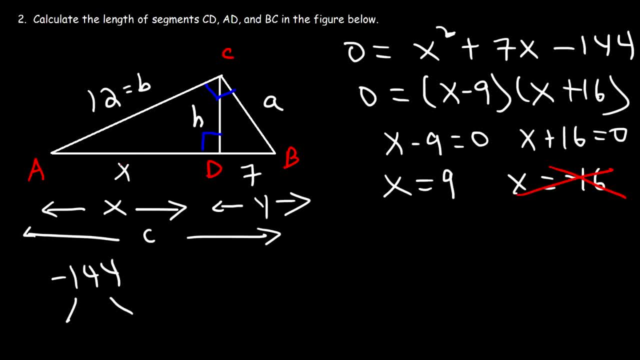 16. Now we can't use this answer because AD cannot be a negative side length, So therefore x has to be positive 9.. So now we know this value. This is 9.. So now we can calculate everything else once we have these two values. 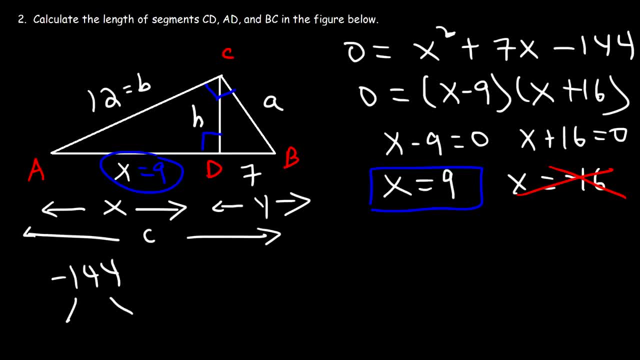 So now we can calculate everything else once we have these two values. So now let's calculate h. So we said that h is the geometric mean between x and y, So it's the square root of x times y, So x is 9 and y is 7.. 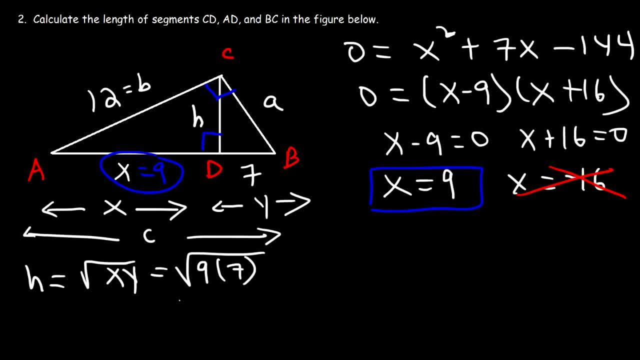 So 9 times 7 is 63,, but we don't have to worry about that. We can take the square root of 9,, which is 3.. So 9 times 7 is 63,, but we don't have to worry about that. 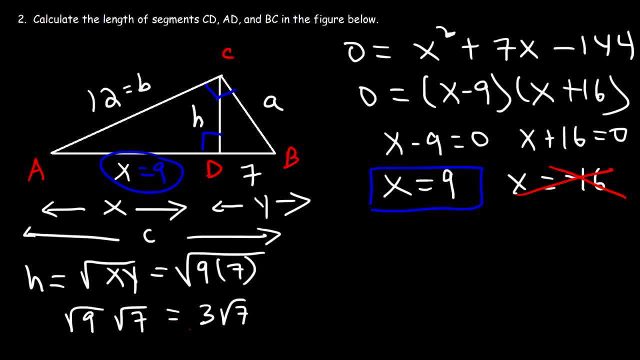 We can take the square root of 9, which is 3.. So h is 3 square root 7.. So we have a simplified radical. Now let's calculate a. So a is the geometric mean between y and c. So a is the square root of y times c. 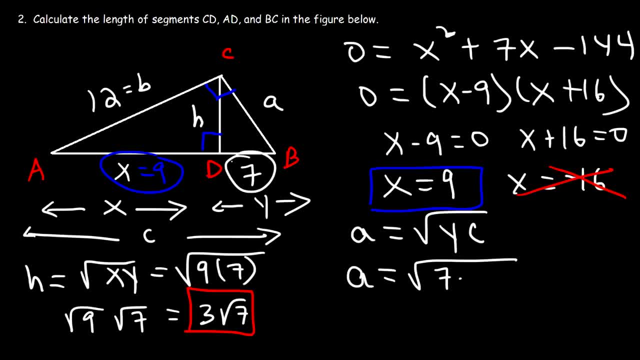 Y in this example is 7. And c is 7 plus 9, or 16.. So h is 3 square root 7.. So we have a simplified radical. Now let's calculate a. Now 16 is a perfect square. 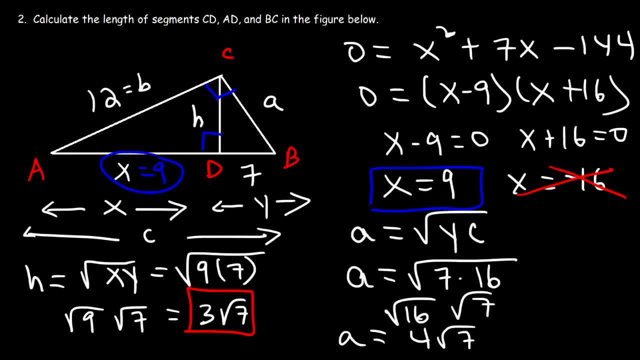 The square root of 16 is 4.. So a is 4 square root 7.. So a represents segment BC and h is segment CD and x is segment AD. So now we have the value of all three segments. AD is 9.. 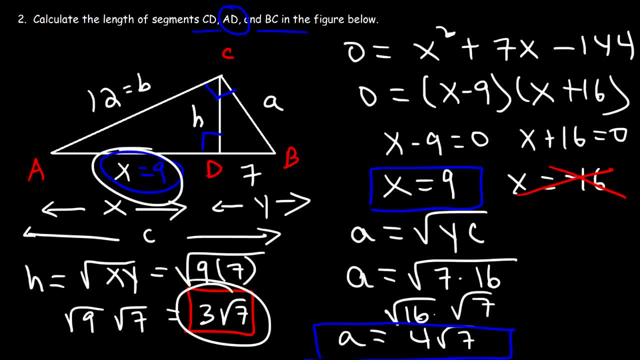 CD is 3 root, 7. And CB or BC is 4.. So we have the value of all three segments: AD is 9.. CD is 3 root, 7. And CB or BC is 4.. So that's it for this problem. 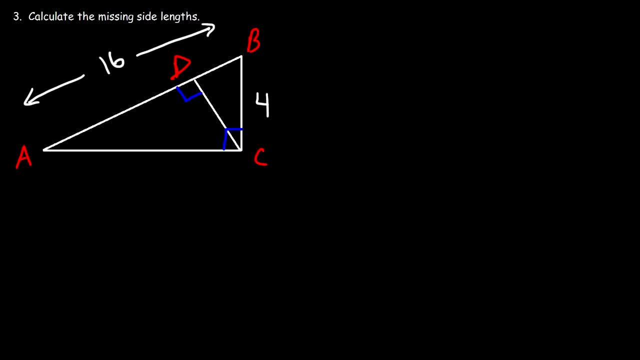 Now let's work on this problem, Calculate the missing side. lengths C and D are always associated with the hypotenuse of this type of triangle. So we have the same triangle as before, but it's simply flipped. Now side A is across angle A. 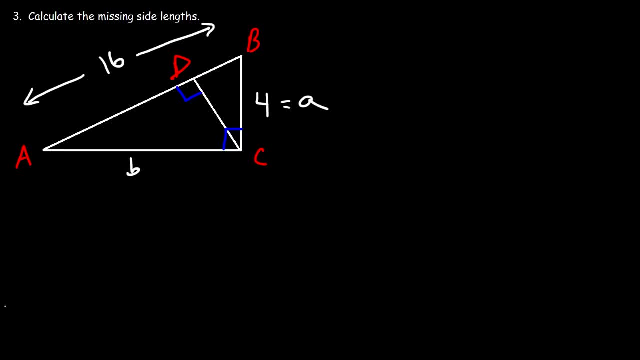 And side B is across angle B, And we know that AD is x, DB is y, And so C is the sum of x and y. So in this example, C is 16. And A is 4. So how can we calculate everything else? 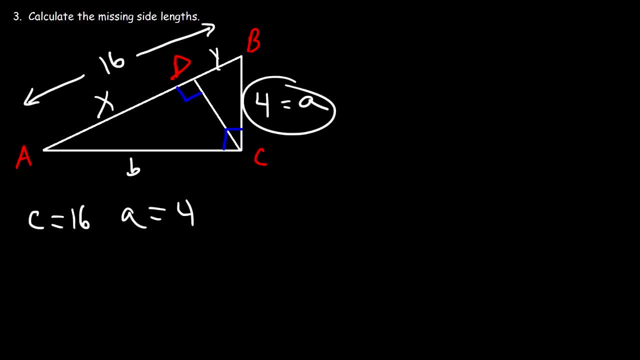 Well, for one thing, remember that A is the geometric mean between C and Y. So A is the geometric mean between C and Y. So C is 16. And A is 4.. So a is the square root of yc. So we have a, which is four. 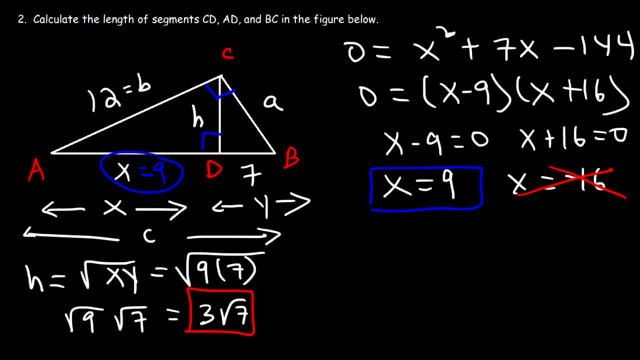 h is 3 square root 7.. So we have a simplified radical. Now let's calculate A. So A is the geometric mean between Y and C. So A is the square root of Y times C. Y in this example, is 7, and C is 7 plus 9, or 16.. 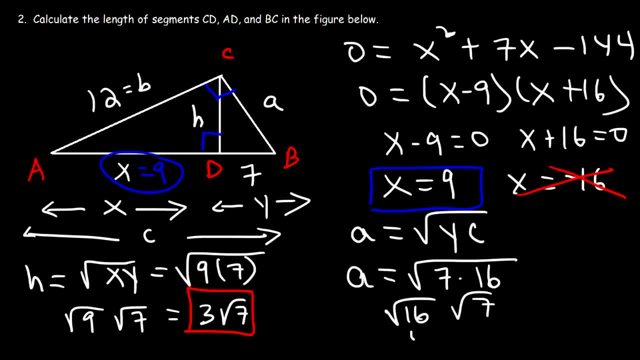 Now 16 is a perfect square. Remember, the square root of 16 is 4.. So A is 4 square root 7.. So A represents segment BC and H is segment CD and X is segment AD. So now we have the value of all three segments. 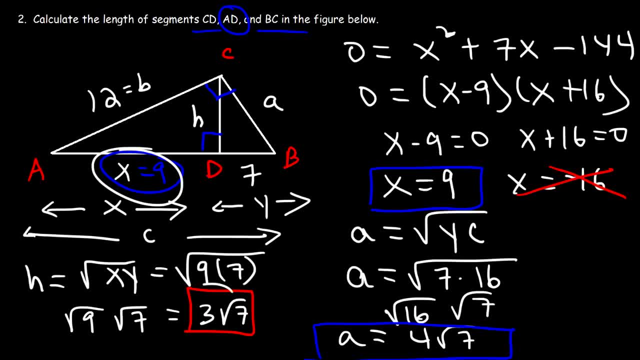 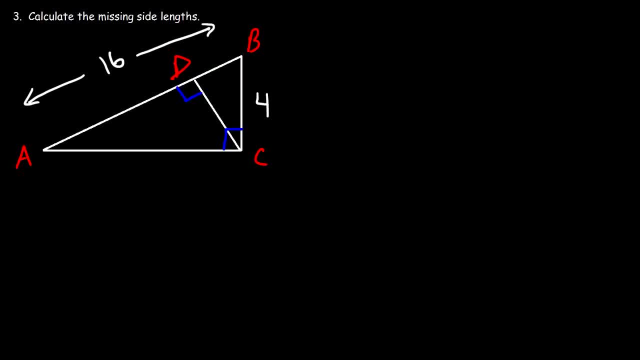 AD is 9,, CD is 3 root 7, and CB or BC is 4 square root 7.. So that's it. So that's it for this problem. Now let's work on this problem. Calculate the missing side lengths. 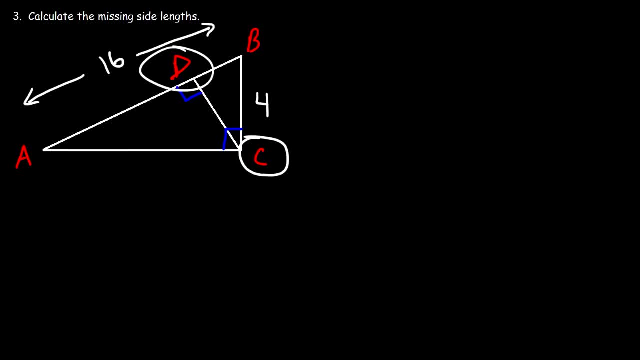 C and D are always associated with the hypotenuse of this type of triangle. So we have the same triangle as before, but it's simply flipped. Now side A is across angle A and side B is across angle B, And we know that AD is X, DB is Y, and so C is the sum of X and Y. 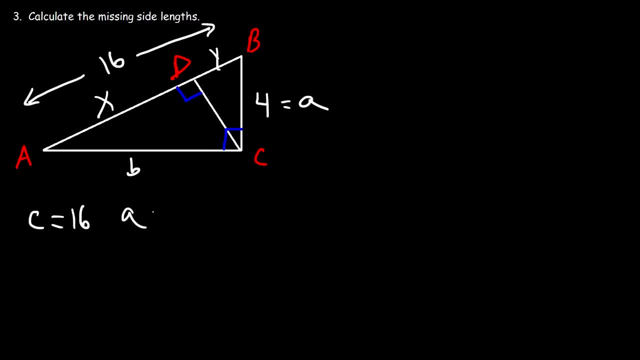 So in this example, C is 16, and A is 4.. So how can we calculate everything else? Well, for one thing, remember that A is the geometric mean between C and Y, So A is the square root of 16.. 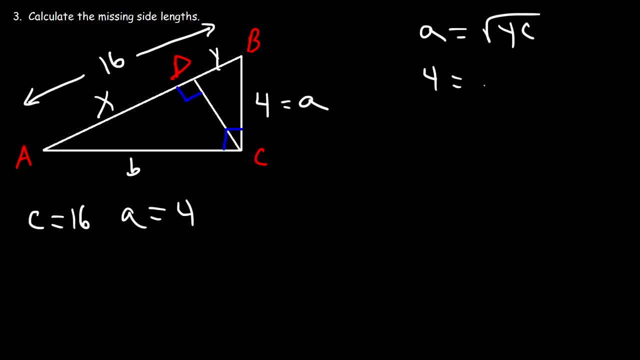 Y is the square root of 16.. So we have A, which is 4, and we have C, that's 16.. So we can calculate Y. So let's square both sides: 4 squared is 16, and once we square the other side, it's going to be just 16Y. 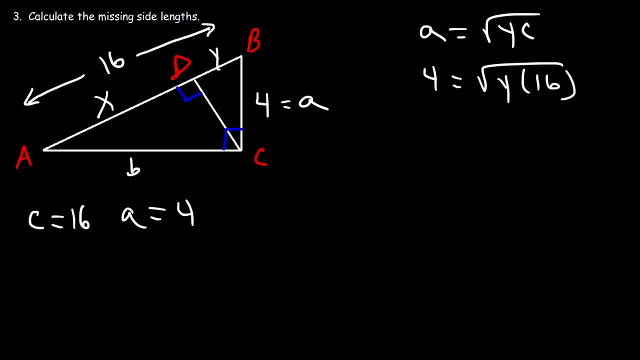 and we have c, that's 16.. So we can calculate y. So let's square both sides. Four squared is 16, and once we square the other side it's gonna be just 16y. So in this example, y is equal to one. 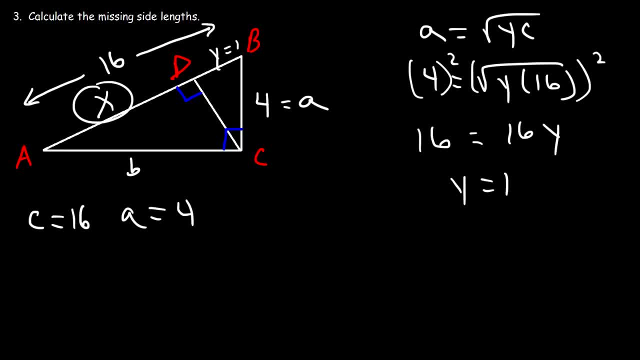 So, if this is one, we can now calculate: x So c is the sum of x plus y, So x is the difference between c and y, So it's 16 minus one, which is 15.. Now, once we have x and y, 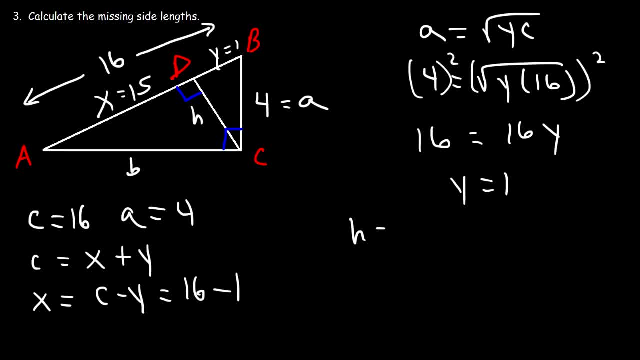 we can easily calculate everything else. So recall that h, the altitude, is the geometric mean between these two values, between x and y. So that's gonna be the square root of 15 times one, and that's simply the square root of 15.. 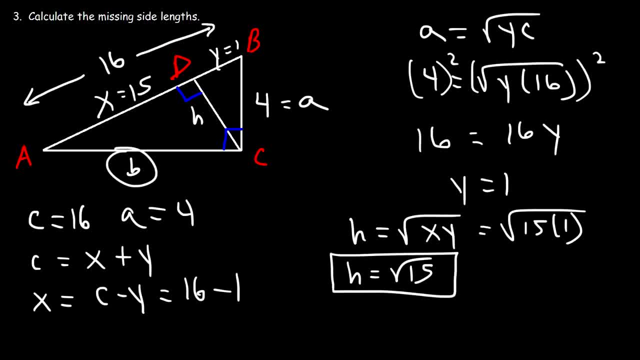 We can't simplify this expression. And b is the geometric mean between x and c, So b is going to be the square root of xc. X is 15 and c is 16.. Now the square root of 16 is four, so it's gonna be four square root of 15.. 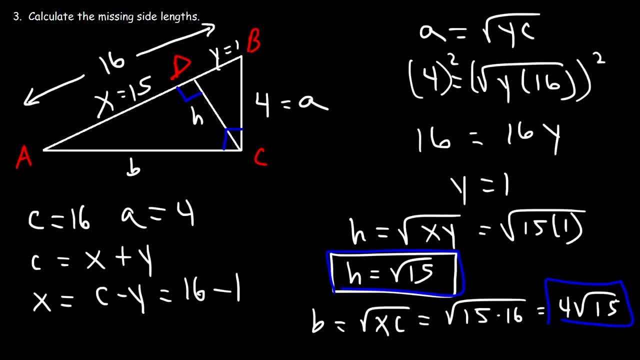 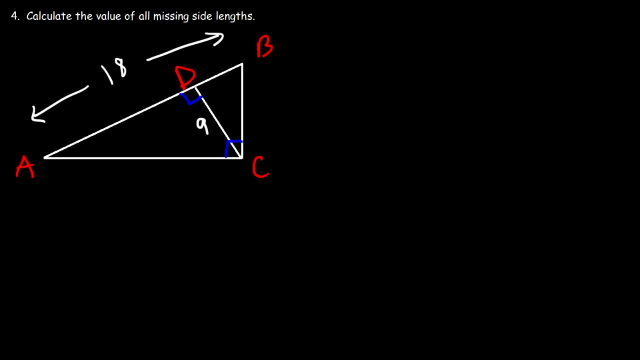 And so that's the value of b. So now we have the value of all the values. So now we have the value of all the values. So now we have the value of all the other missing sides. Go ahead and try this problem. 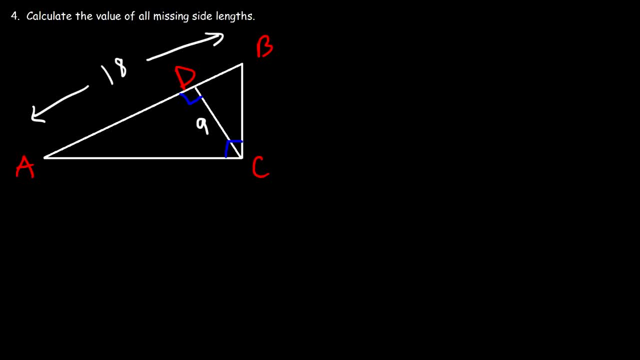 Let's calculate the value of all the missing sides. So we know that a is a cross angle a, So this is side a. B is a cross angle b And ad is x, Db is y And c is ab. So in this example we have c, which is 18,. 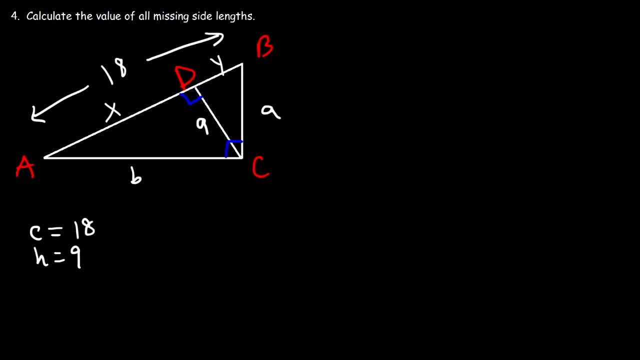 and h, which is nine. Now it turns out that whenever h is one half of c, x, y and h are all equal to each other. x, y and h are all equal to each other, So x and y is nine. 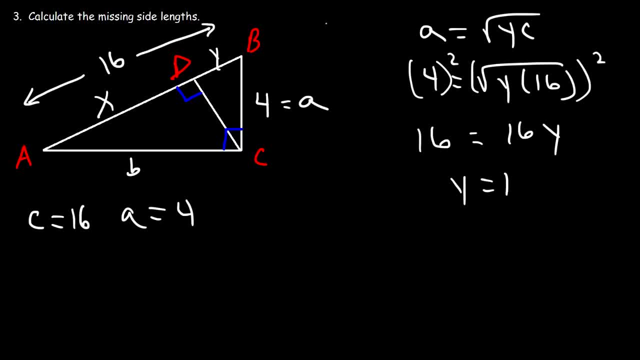 So in this example, Y is equal to 1.. So if this is 1, we can now calculate: Y So C is the sum of X plus Y, So X is the difference between C and Y. So it's 16 minus 1, which is 15.. 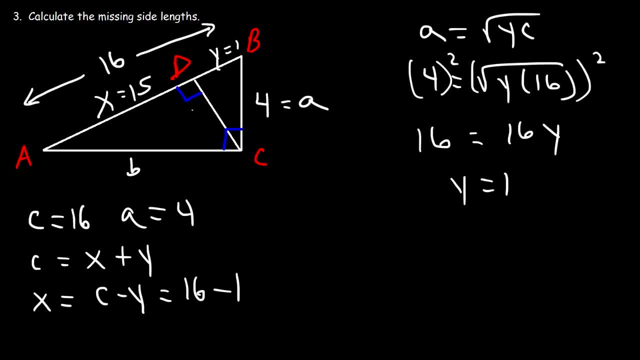 Now, once we have X and Y, we can easily calculate everything else. So recall that H, the altitude, is the geometric mean between these two values, between X and Y. So that's going to be the square root of 15 times 1,. 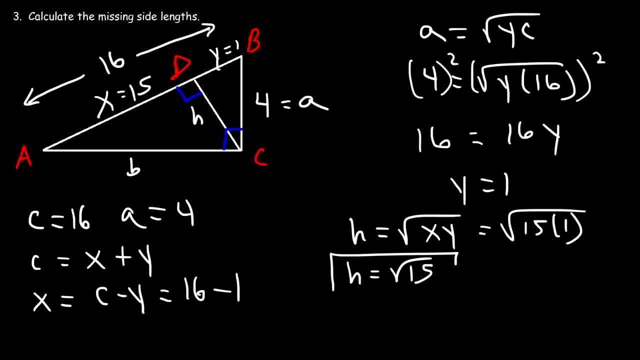 and that's simply the square root of 15.. We can't simplify this expression. And B is the geometric mean between X and C, So B is going to be the square root of XC. X is 15, and C is 16.. 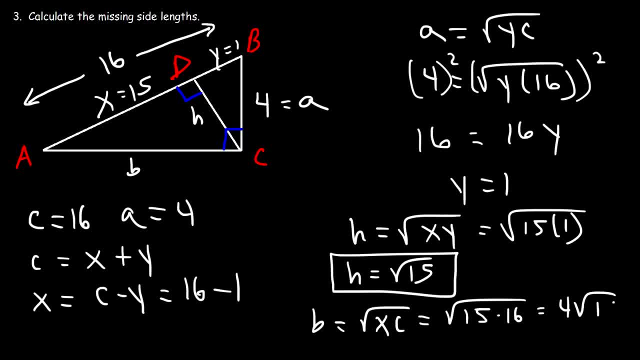 Now the square root of 16 is 4, so it's going to be 4 squared root of 15.. And so that's the value of B. So now we have the value of all the other missing sides. Go ahead and try this problem. 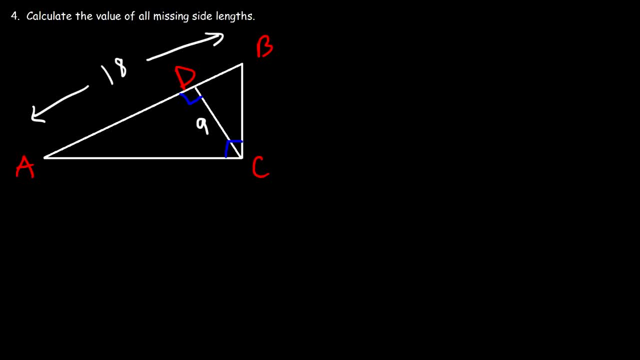 Let's calculate the value of all the missing sides. So we know that A is across angle A, so this is side A, B is across angle B And AD is X, DB is Y and C is AB. So in this example we have C, which is 18, and H, which is 9.. 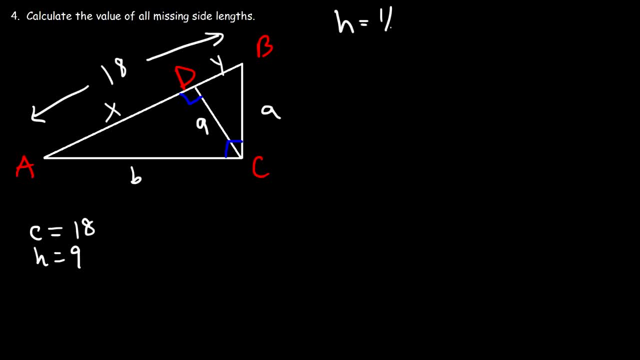 Now it turns out that whenever H is one-half of C, X, Y and H are all equal to each other, So X and Y is 9.. Now let's confirm this. So what formulas can we use? We know that H is the geometric mean between X and Y. 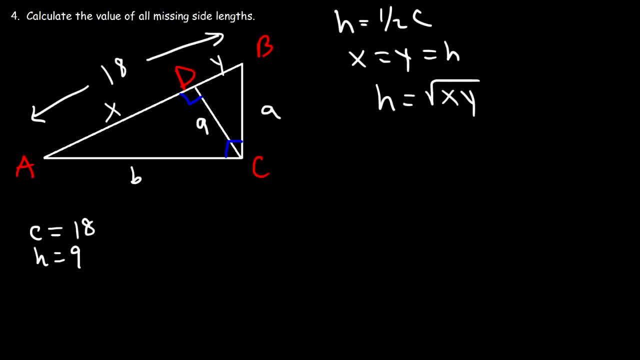 So H is equal to the square root of X and Y, And H is 9, so we have this formula. Now also notice that C is the sum of X and Y, So we can say that 18 is equal to X plus Y. 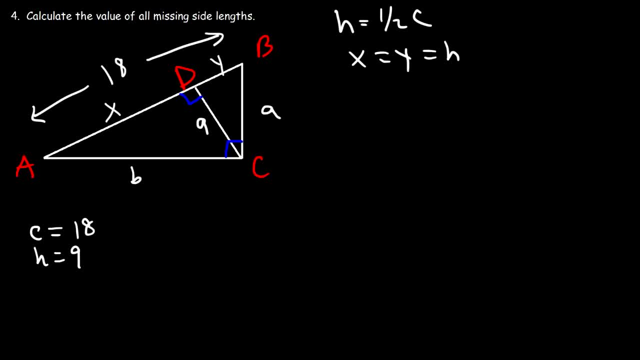 Now let's confirm this. So what formulas can we use? We know that h is the geometric mean between x and y, So h is equal to the square root of x and y, And h is nine. so we have this formula. Now also notice that c is the sum of x and y. 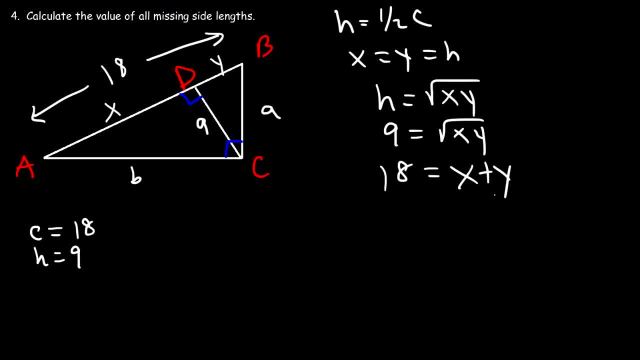 So we could say that 18 is equal to x plus y. So we have two equations and two variables. So we could solve it using a system of equations. Let's go ahead and square this side. Nine squared is 81, and that's equal to x times y. 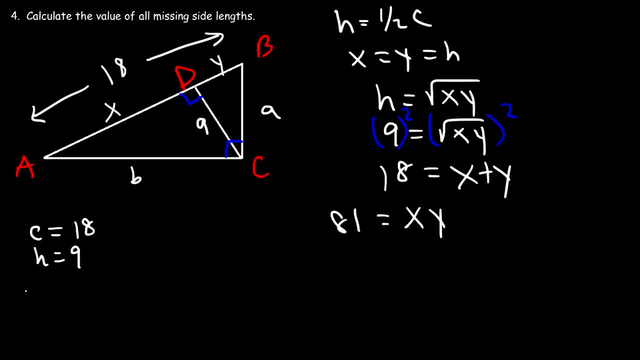 In this equation let's isolate y, So we need to subtract both sides by x. 18 minus x is y, And so let's replace y with this. So 81 is equal to x times 18 minus x. Now what is the value of x? 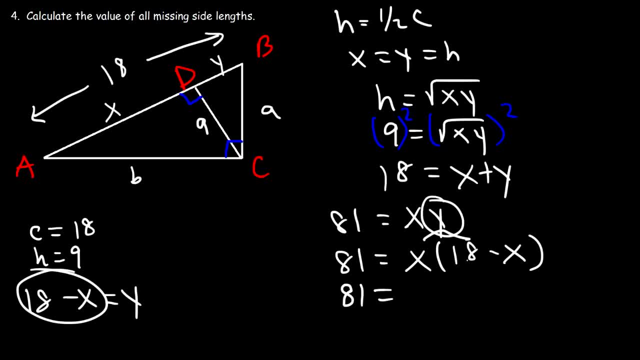 So let's distribute x first. So x times 18 is 18x. X times negative x is negative x squared. Let's take everything on the right side and move it to the left side, So negative x squared on the right becomes positive x squared on the left. 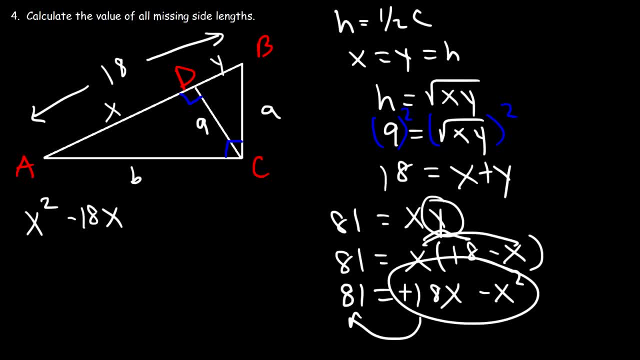 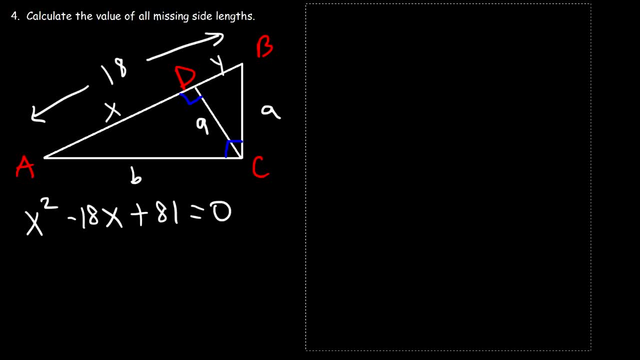 Positive 18x on the right becomes negative 18x on the left And 81 is still on the left, so it's gonna remain positive. Now what two numbers multiply to positive 81 but add to negative 18? This is gonna be negative nine and negative nine. 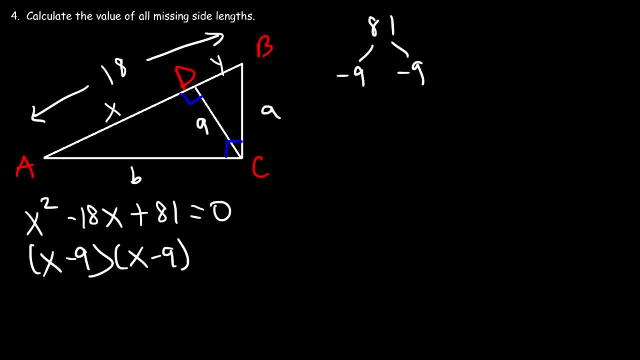 So we can factor in, say x minus nine times x minus nine, Or simply x minus nine squared, If we take the square root of both sides. the square root of x minus nine squared is x minus nine. Square root of zero is zero. 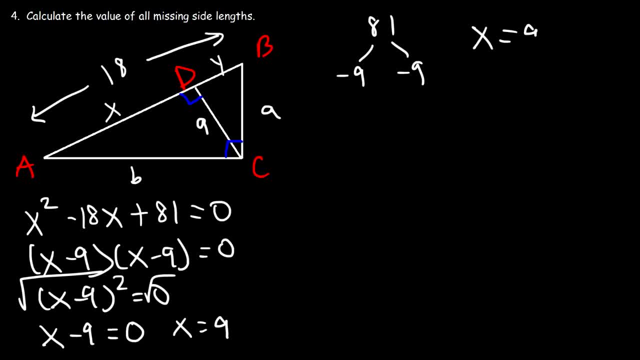 And so if we add nine to both sides, we can see that x is nine. Now c is x plus y And c is 18.. So if x is nine, then y has to be 18 minus nine, which is nine as well. 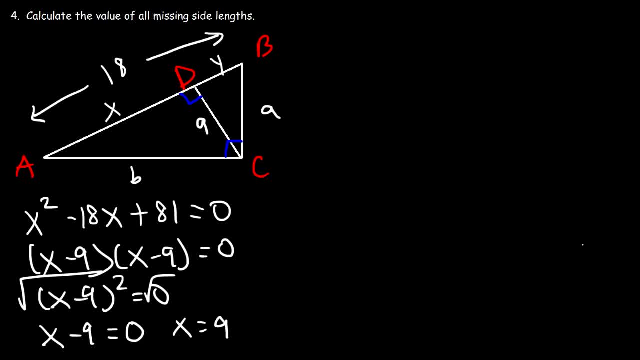 So whenever h is one half of c, so whenever this number is half of this number, x and y are both equal to this number. So knowing that fact can help you to solve a problem like this quickly. So now we can calculate the value of a and b. 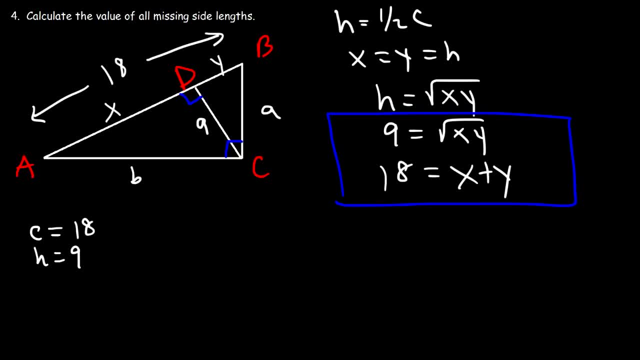 So we have two equations and two variables, So we could solve it using a system of equations. Let's go ahead and square this side: 9 squared is 81, and that's equal to X times Y. In this equation, let's isolate Y. 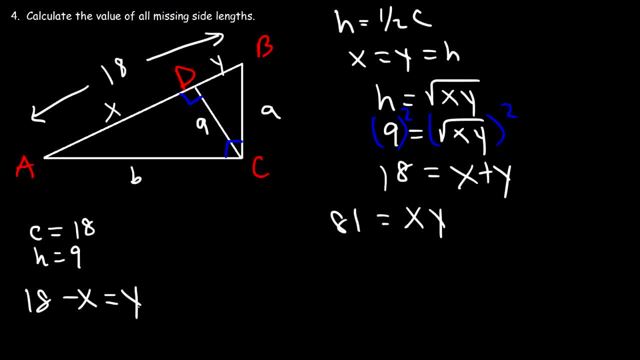 So we need to subtract both sides by X. 18 minus X is Y, And so let's replace Y with this. So 81 is equal to X times 18 minus X. Now what is the value of X? So let's distribute X first. 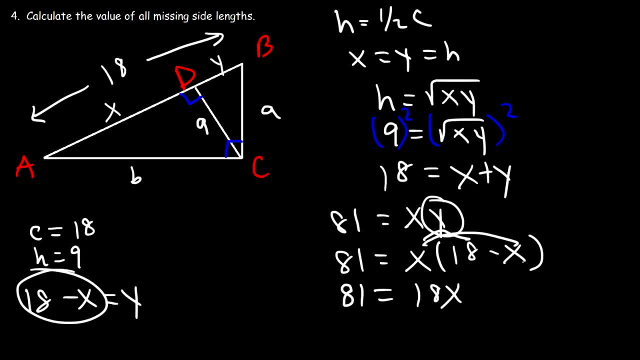 So X times 18 is 18X. X times negative X is negative X squared. Let's take everything on the right side and move it to the left side, So negative X squared on the right becomes positive X squared on the left. 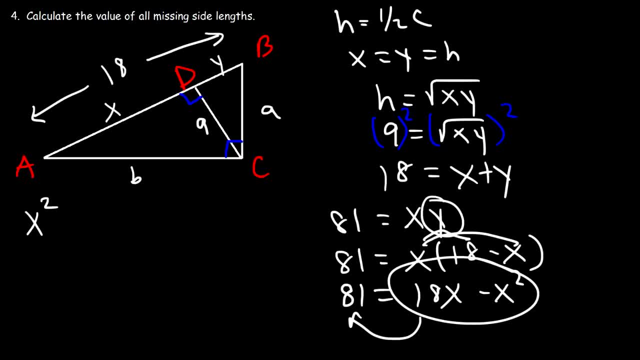 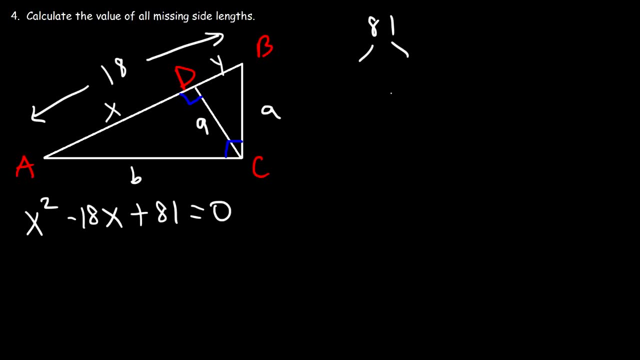 Positive 18X on the right becomes negative 18X on the left, And 81 is still on the left, so it's going to remain positive. Now, what two numbers multiply to positive 81, but add to negative 18? This is going to be negative 9 and negative 9.. 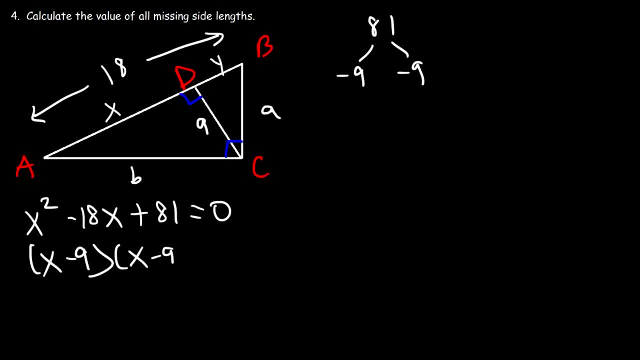 So we can factor and say X minus 9 times X minus 9.. Or simply X minus 9 squared. If we take the square root of both sides, we get negative 9.. The square root of X minus 9 squared is X minus 9.. 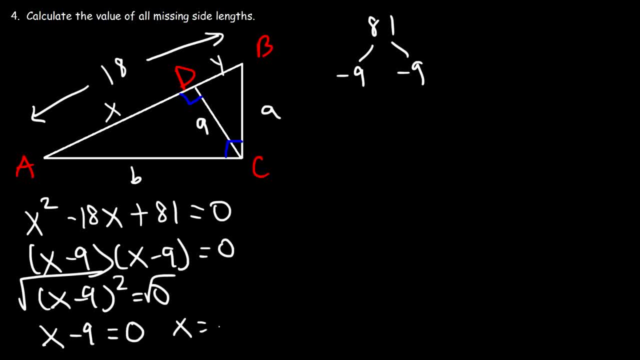 The square root of 0 is 0. And so if we add 9 to both sides, we can see that X is 9.. Now C is X plus Y And C is 18.. So if X is 9, then Y has to be 18 minus 9,. 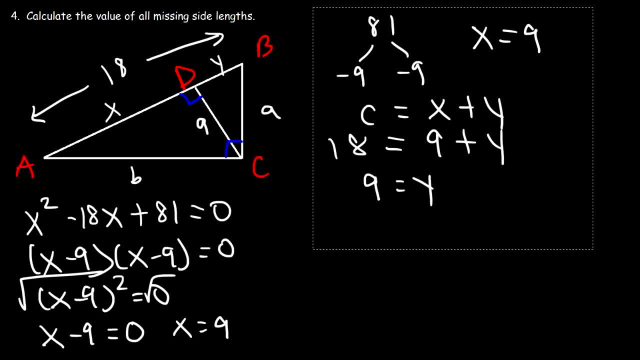 which is 9 as well. So whenever H is one half of C, so whenever this number is half of this number, X and Y are both equal to this number. So knowing that fact can help you to solve a problem like this quickly. 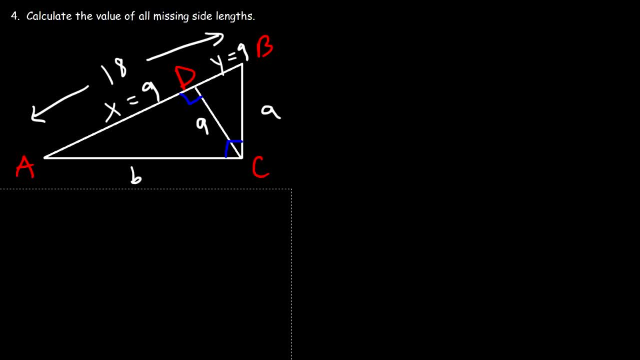 So now we can calculate the value of a and b. So we know that a is the geometric mean of Y and C. So a is the square root of YC And Y is 9.. C is 18.. And so 9 times 18.. 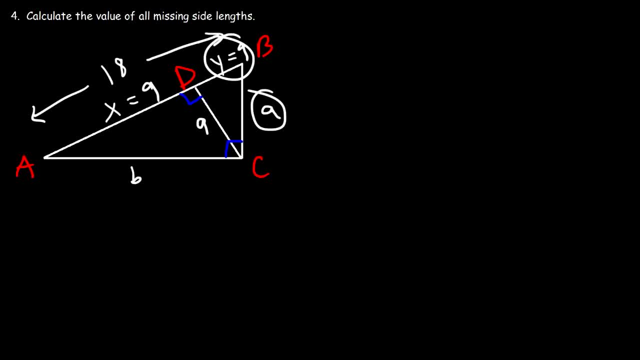 So we know that a is the geometric mean of y and c. So a is the square root of yc And y is nine, C is 18.. And so nine times 18 is 162.. And 162 is 81 times two. 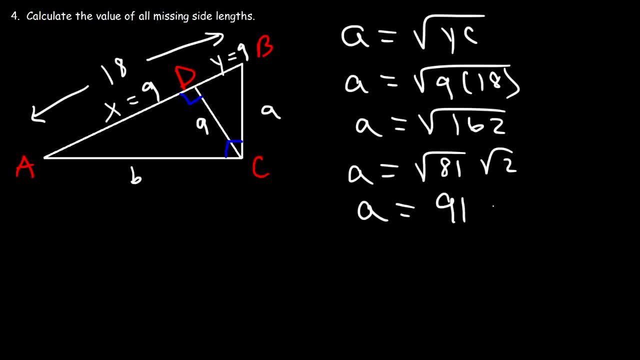 81 is the perfect square And the square root of 81 is nine, So that's the value of a. I wrote 91 for some reason, So a is nine, square root two. Now b is the geometric mean of x and c. 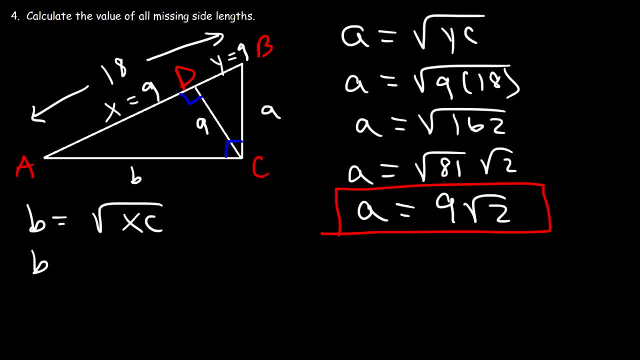 In this case, x is nine and c is still 18, which will give us the same answer as a. So it's nine square root two. So notice that both a and b is equal to whatever x and y is times the square root of two. 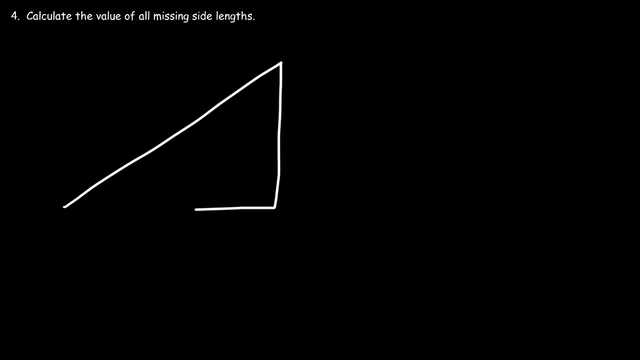 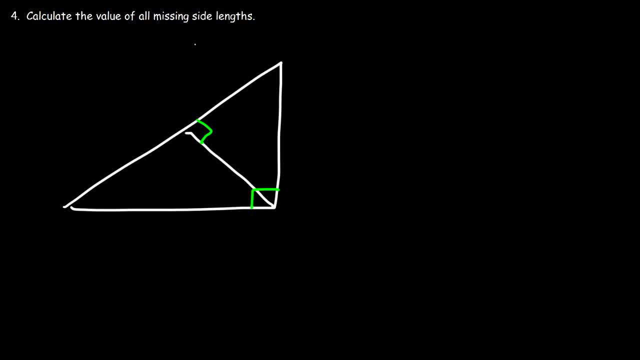 So let's say, if we have the same figure And let's say c is 16, And let's say this is eight, So notice that h is one-half of c. So automatically you know this is eight, this is eight, And two sides are eight, square root two. 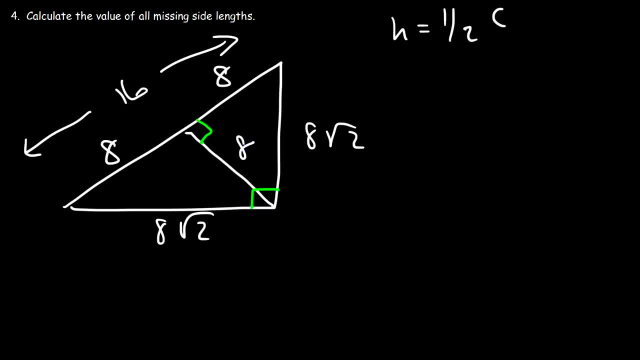 And that's it. if you know that this is one-half of this value, Here's the last problem. So, given this, Between the value of a and b, how can we find everything else? So how can we find the value of x, y, h and also c? 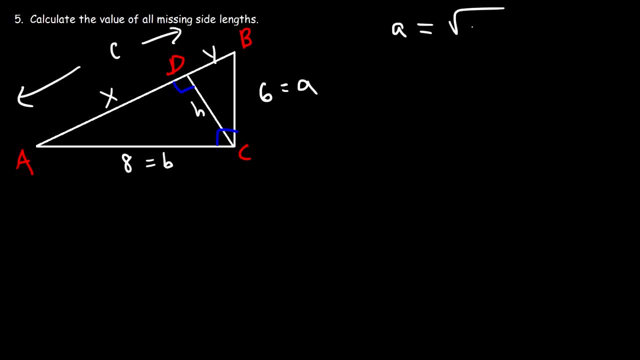 Now we know that a is the geometric mean between y and c. Now we don't know the value of y or c, so that's not going to be useful to us. And b is the geometric mean between x and c. So we don't have those values, so that's not helpful. 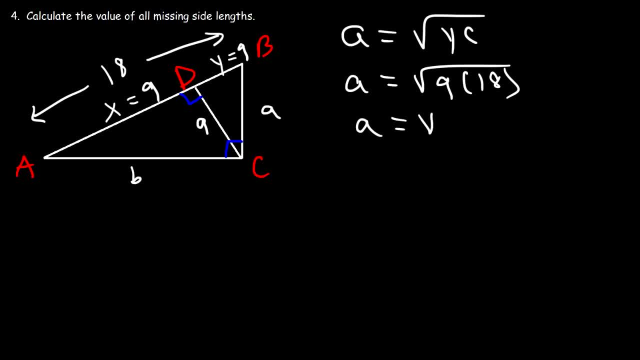 S is 9.. We know C is 18.. is 162. And 162 is 81 times 2.. 81 is a perfect square And the square root of 81 is 9.. So that's the value of A. I wrote 91 for some reason, So A is 9 square root 2.. Now B is: 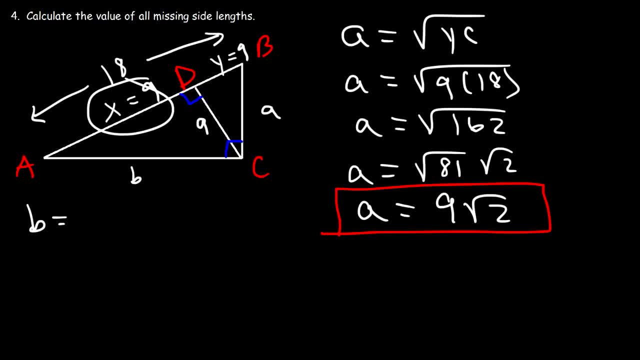 the geometric mean of X and C. In this case, X is 9 and C is still 18,, which will give us the same answer as A. So it's 9 square root 2.. So notice that both A and B is equal. 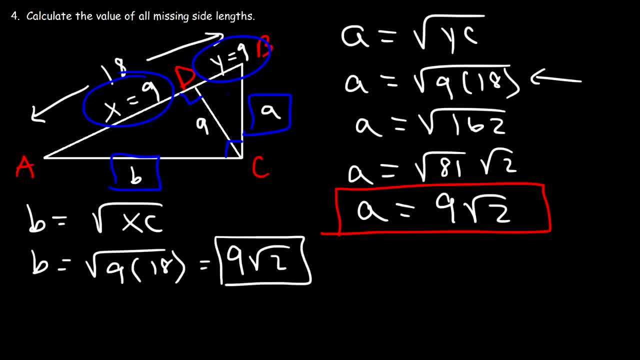 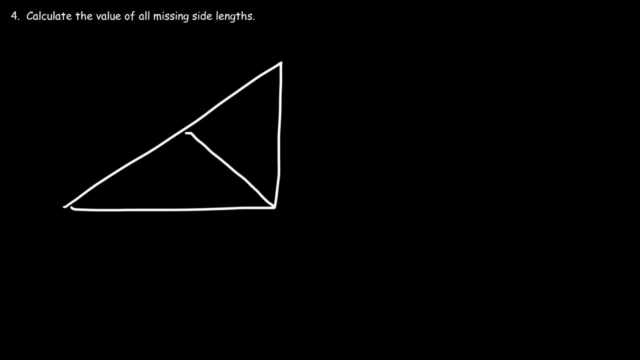 to whatever X and Y is times the square root of 2.. So let me give you an example problem. So let's say, if we have the same figure And let's say C is 16.. And let's say this is 8.. So notice that H is one half of C. So 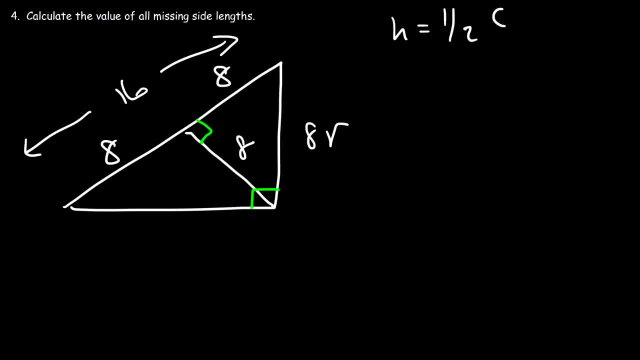 automatically. you know, this is 8, this is 8. And these two sides are 8, square root 2.. And that's it. If you know that this is one half of this value, Here's the last problem. So, given the value of A and B, how can we find everything else? So how can we find the? 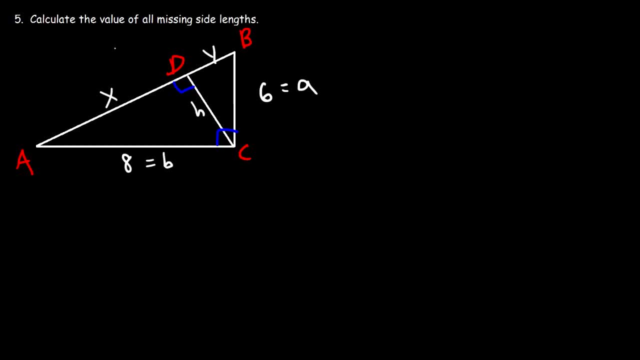 value of X, Y, H and also C. Now we know that A is the geometric mean between Y and C. Now we don't know the value of Y or C, so that's not going to be useful to us. And B is the. 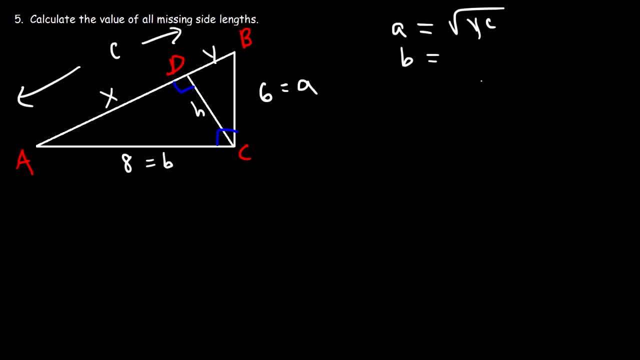 geometric mean between X and C, So we don't have those values, so that's not helpful. And H is the geometric mean between X and Y. We have none of those values, So that's not useful either. So how can we solve this thing if none of these equations are helpful? 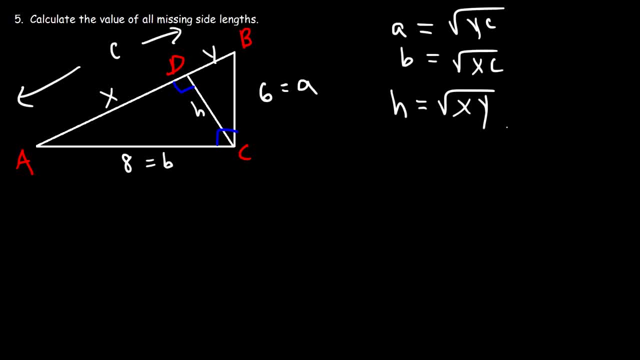 at this point. Now, if we try to write a system of equations, let's say 6 is equal to the square root of YC, Which is 8, that's equal to the square root of XC. We have three missing variables Now. 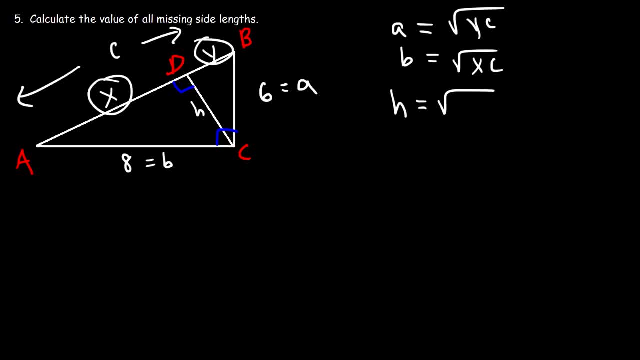 And h is the geometric mean between x and y. We have none of those values, so that's not useful either. So how can we solve this thing if none of these equations are helpful at this point? Now, if we try to write a system of equations, let's say 6 is equal to the square root of 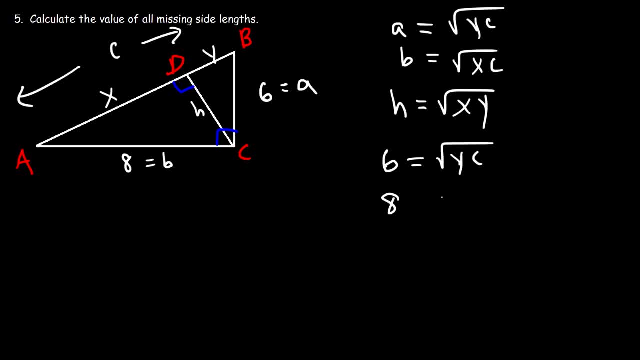 yc, Okay, And b, which is 8,, that's equal to the square root of xc. We have three missing variables Now. granted, we could replace c with x plus y in both equations, And so now we have two equations with two variables. 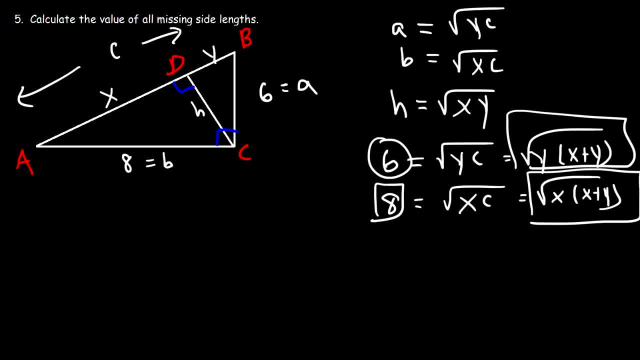 So technically, we could solve this, but I think that's going to be a lot of work, So let's avoid that and let's find an easier way Now. there are some other equations that you could use besides these three. So if you focus on the large triangle, notice that it's a right triangle. 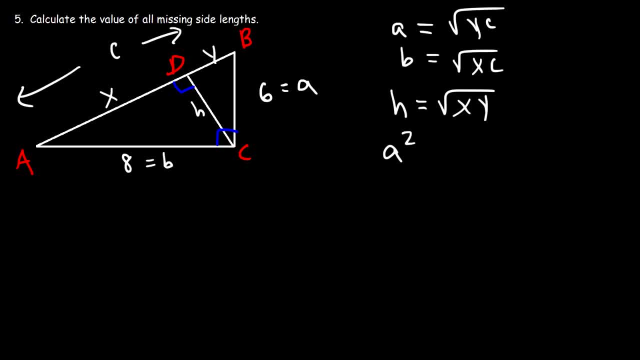 So we can use the Pythagorean Theorem. So for that triangle, a squared plus b squared is equal to c squared. Now let's focus on this triangle. This is also a right triangle. So we have this formula: x squared plus a squared is equal to the hypotenuse for that. 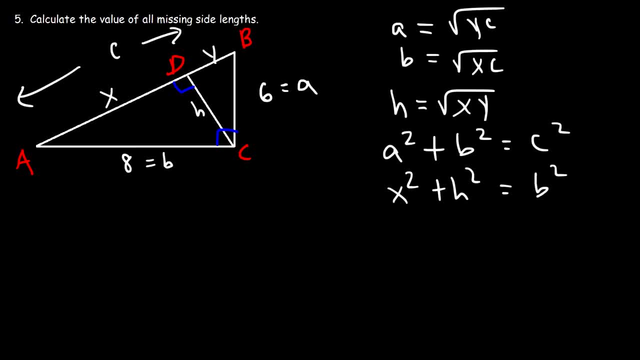 triangle Which is b squared. Well, the hypotenuse is b, but this formula is equal to b squared. Now, if we focus on this triangle, the hypotenuse is a, So thus y squared plus h squared is equal to a squared. 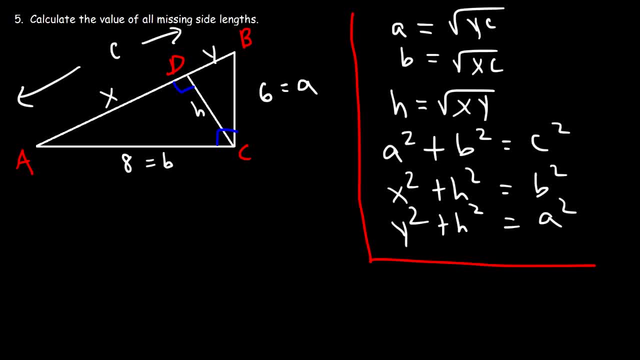 So these are the six formulas that are useful for this type of problem, This altitude on hypotenuse situation. Now let's use this equation to calculate c. So a is 6, b is 8, and let's find c: 6 squared is 36,. 8 times 8 is 64.. 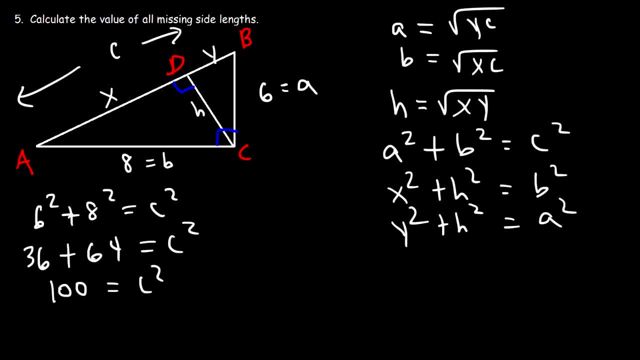 36 plus 64 is 100.. And the square root of 100 is 10.. So c is equal to 10.. So I'm going to just put this here. So, now that we have the value of c and ab, We can use these two equations. 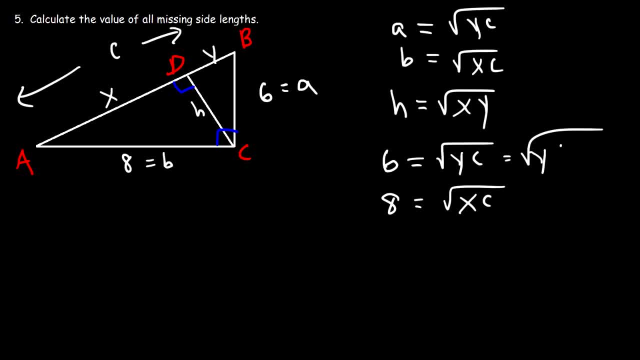 granted, we could replace C with X plus Y in both equations, And so now we have two equations with two variables. So technically we could solve this, but I think that's going to be a lot of work, So let's avoid that and let's find an easier way Now there are 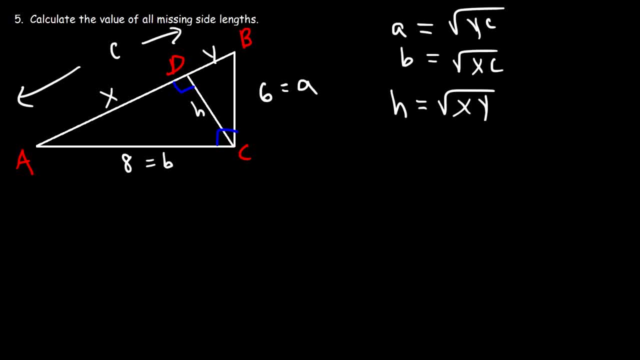 other equations that you could use besides these three. So if you focus on the large triangle, notice that it's a right triangle, So we can use the Pythagorean Theorem. So for that triangle, A squared plus B squared is equal to C squared. Now let's focus on 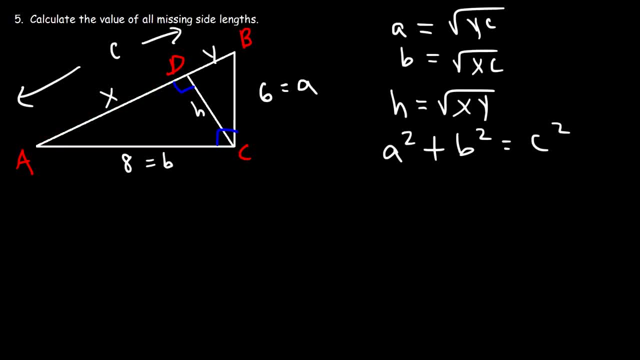 this triangle. This is also a right triangle. So we have this formula: X squared plus A squared is equal to the hypotenuse for that triangle, which is B squared. Well, the hypotenuse is B, but this formula is equal to B squared. Now, if we focus on 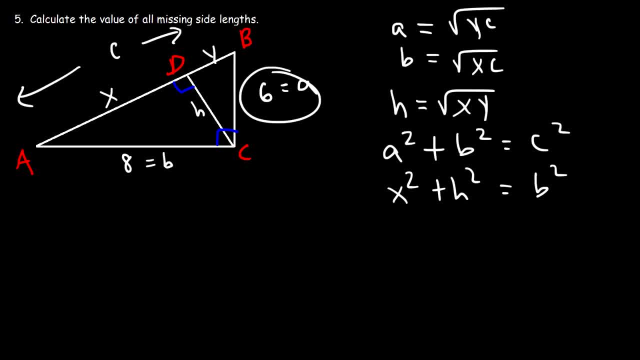 this triangle the hypotenuse is A, So thus Y squared plus H squared is equal to A squared. So these are the six formulas that are useful for this type of problem, this altitude on hypotenuse situation. Now let's use this equation to calculate C. So 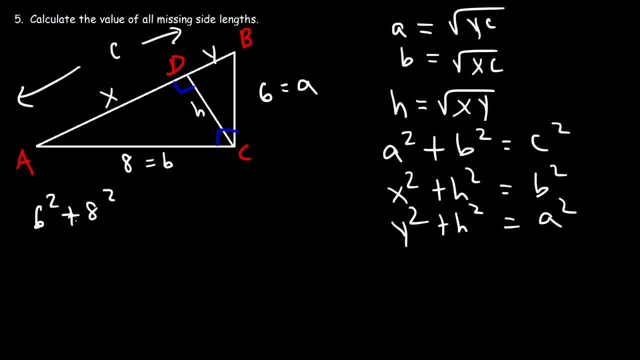 A is 6.. B is 8.. Now let's find C. 6 squared is 36.. 8 times 8 is 64.. 36 plus 64 is 100.. And the square root of 100 is 10.. So C is equal to 10.. So I'm going to just put this here. So now that 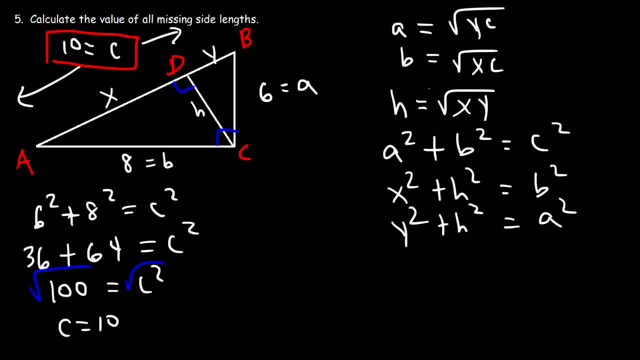 we have the value of C and AB. we can use these two equations to calculate the value of X and Y. So let's start with the value of X. So, using this formula, B is 8 and C is 10.. So let's. 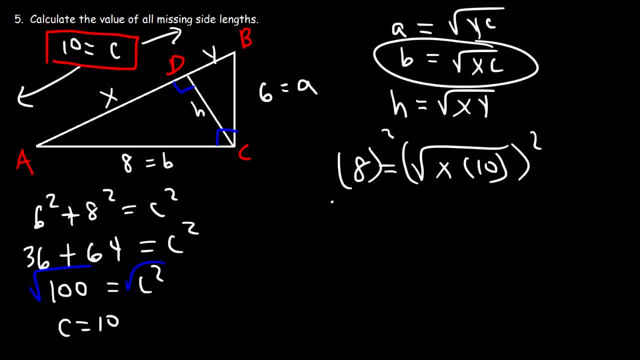 take the square of both sides to get rid of the square root. 8 squared is 64.. And the square and the square root will cancel giving us 10X. So if we divide both sides by 10, we can get the value of X, which in this example is 6.4.. 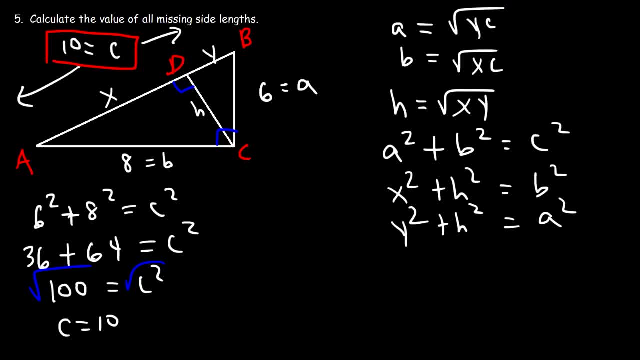 To calculate the value of x and y. So let's start with the value of x. So, using this formula, b is 8 and c is 10.. So let's take the square of both sides to get rid of the square root. 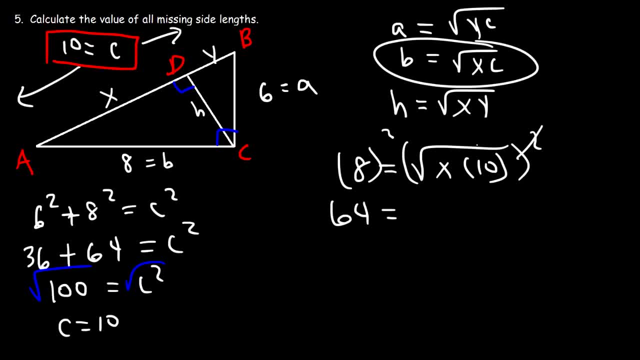 8 squared is 64. And the square and the square root will cancel Giving us 10x. So if we divide both sides by 10. We can get the value of x, Which in this example is 6.4.. 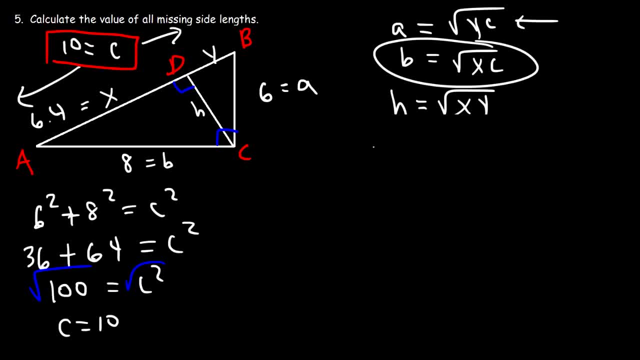 So now we can calculate the value of y And we don't need to use this formula. We know that c is x plus y, And that's another equation you can write down if you want to: C is 10.. X is 6.4.. 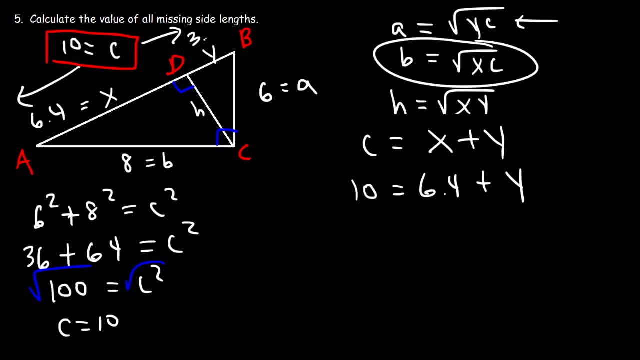 So y is 10 minus 6.4.. Which means y is 3.6.. So we can calculate the value of y And we don't need to use this formula. So now we can calculate the value of h. H is the square root of x- y. 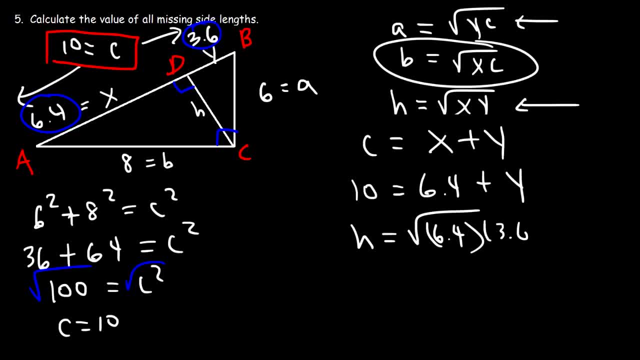 So it's the square root of 6.4 times 3.6.. And I'm definitely going to use a calculator for that. So h is 4.8.. And so that's the answer. Now to verify that we have the right answer. 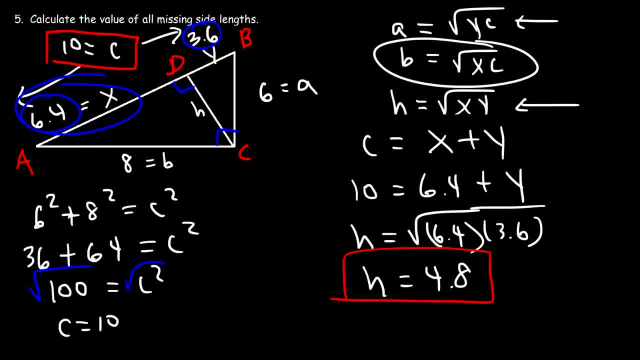 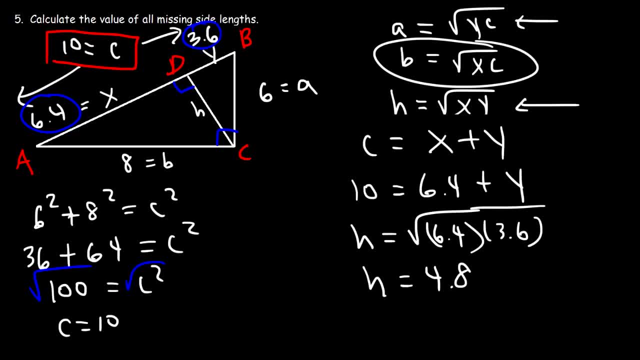 And then for this one, 3.6 squared plus 4.8 squared has to equal a squared which is 36, and that does. So that means that these numbers are correct, and so that's what you can do if you're given. 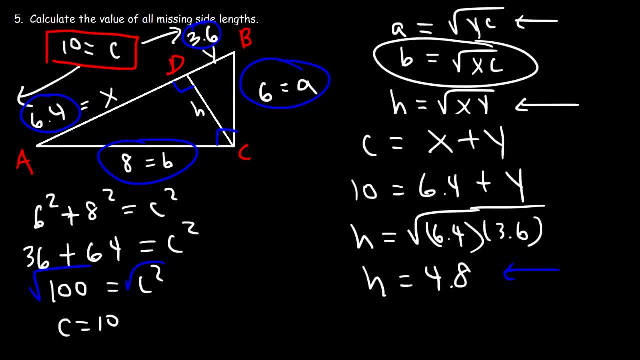 3.6 squared plus 4.8 squared, which is 36, and that does. That's how you can find everything else in this triangle using this process.